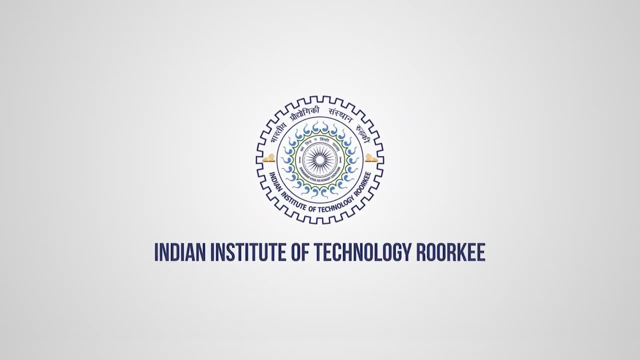 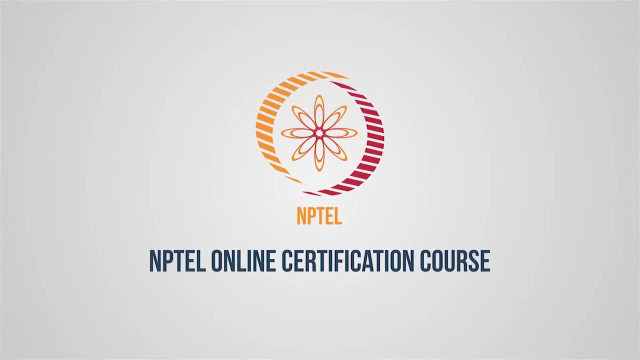 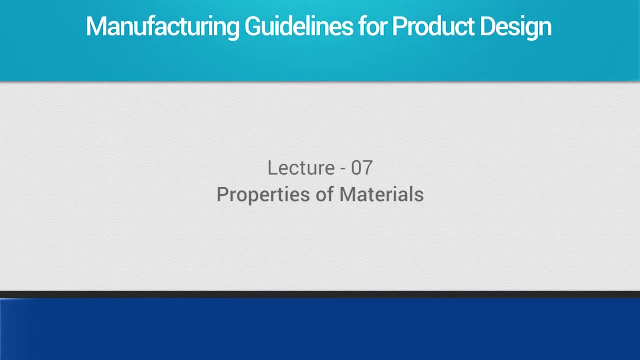 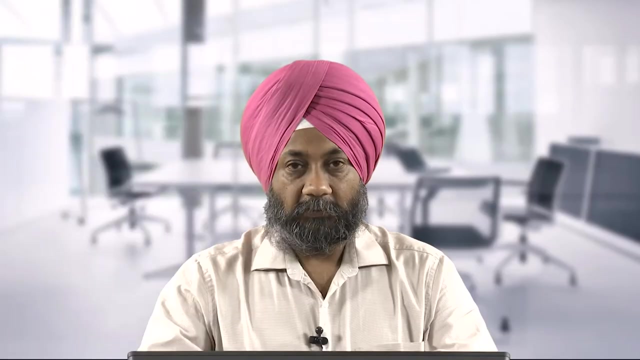 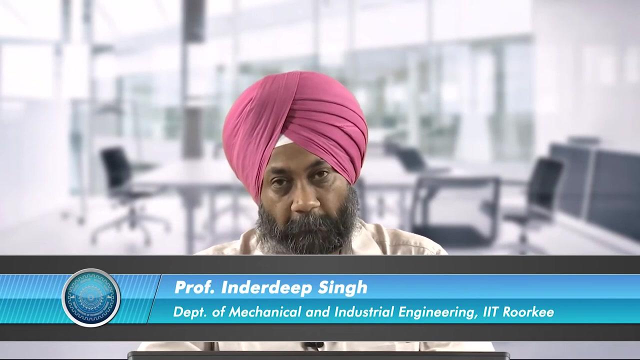 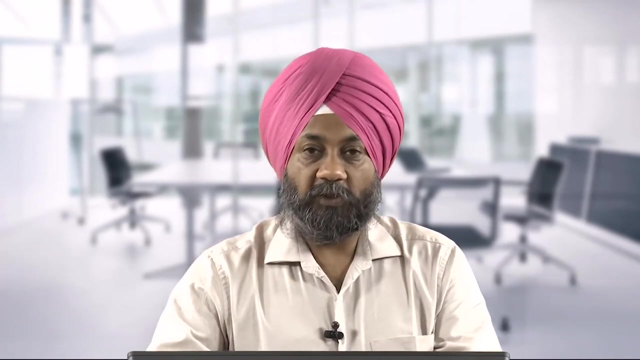 Namaskar friends, welcome to session 7 of our course on Manufacturing Guidelines for Product Design. If we have a quick review of what we have covered till today, we have covered the basic aspects of manufacturing processes, the classification of manufacturing processes, the applications, 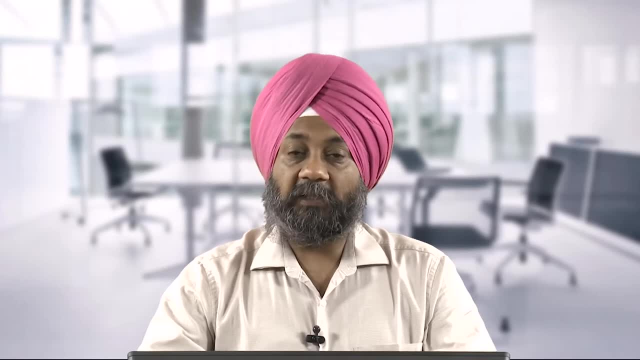 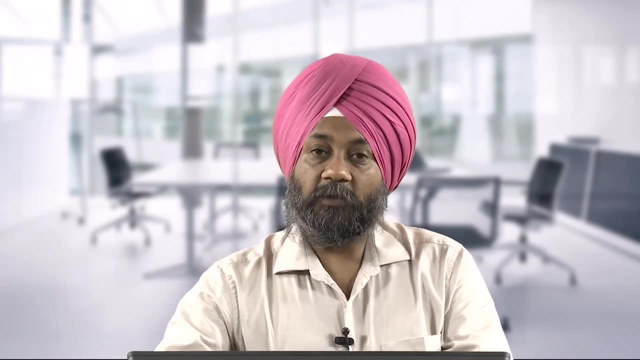 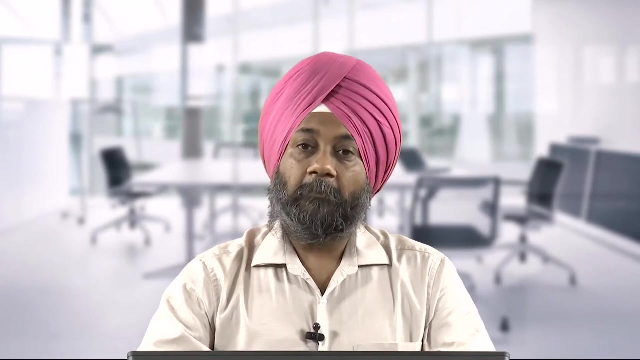 of manufacturing processes and we have tried to see that. what are the process capabilities of the various types of manufacturing processes? We tried to see the application areas of the manufacturing processes, although we have not gone into the details of the manufacturing processes, The manufacturing mechanics of the manufacturing processes or the parameters governing a particular. 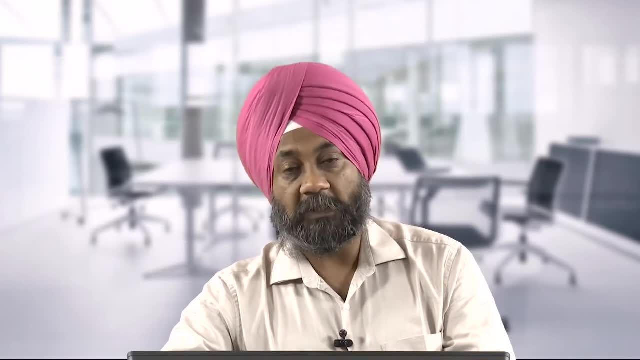 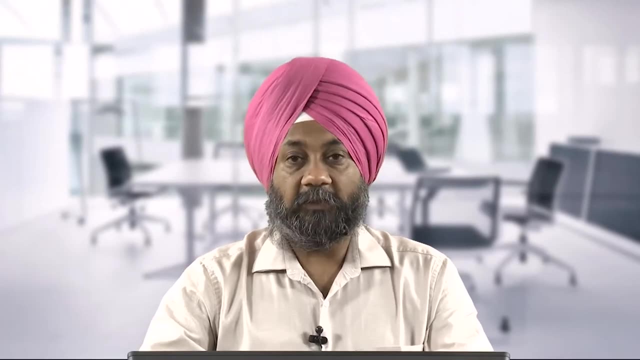 manufacturing process. but we have tried to understand from the application point of view that which process can be used under what type of circumstances, under what type of conditions, And in that we have seen that casting can be used for a very specific application- machining- 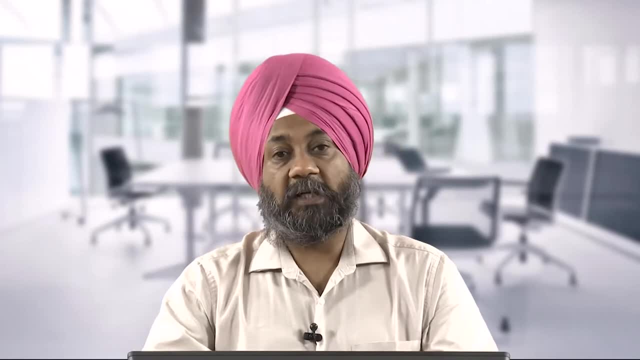 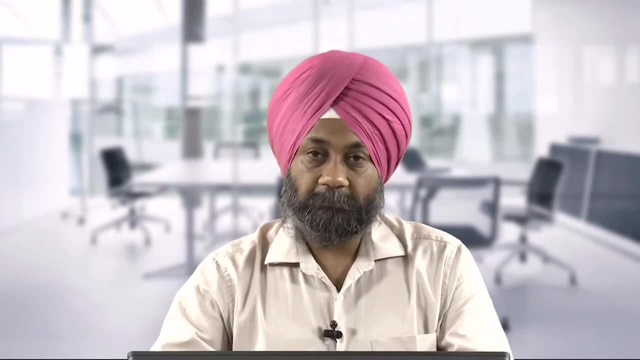 can be used for a specific application, and then we have listed a criteria which will help us to decide that which manufacturing process can be used for which type of manufacturing process. In the second week of our discussion, we started the discussion with introduction to the engineering. 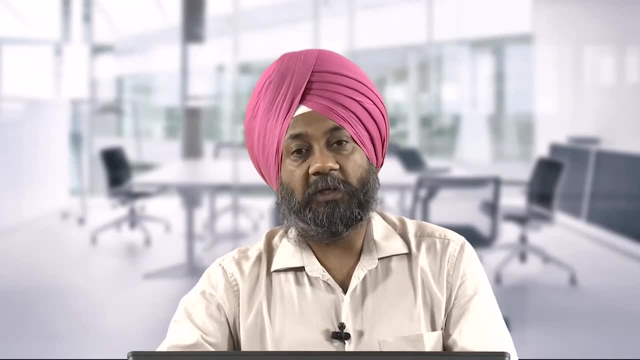 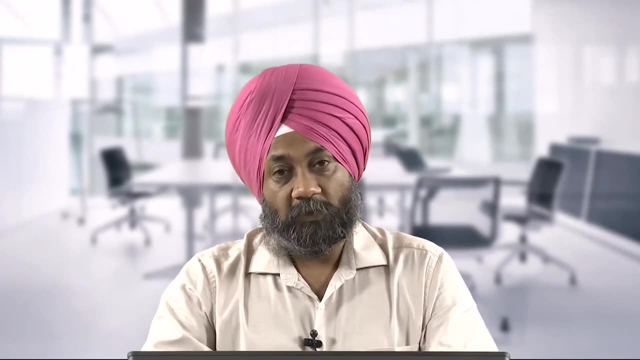 materials in which we have seen. what are the various types of engineering materials that we use If we see all around us, so many types of engineering materials are there. There are polymers, there are plastics. polymers or plastics- one and the same thing. 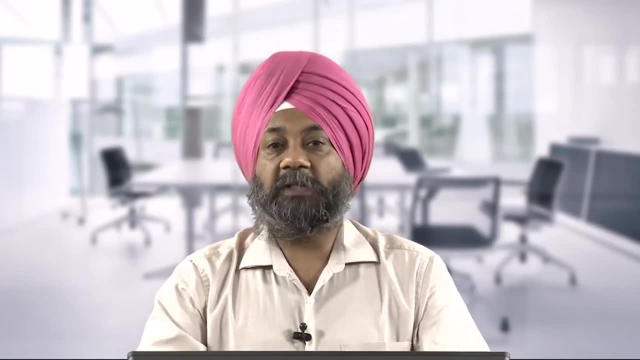 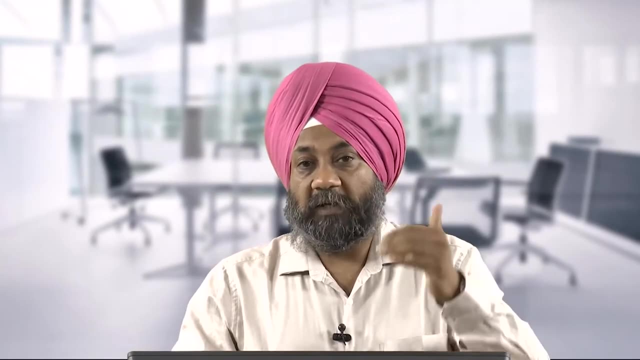 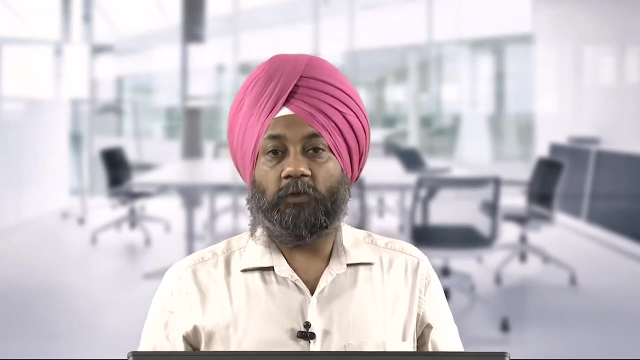 We have metals, we have wood, we have other types of materials like ceramics. so we have tried to classify the engineering materials. We have classified the engineering materials into different classes or different families or different groups. Today our target is to see that what are the properties of the engineering materials which? 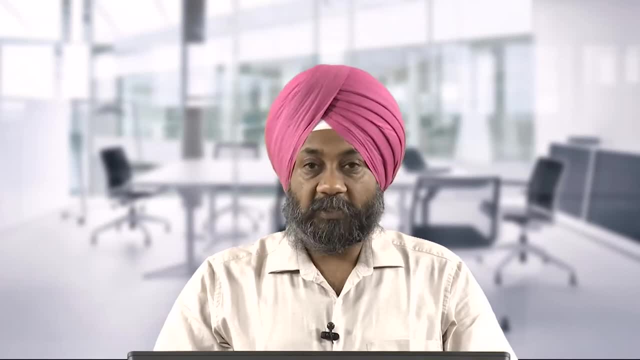 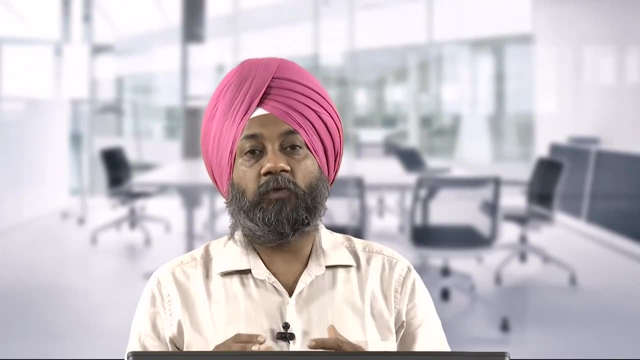 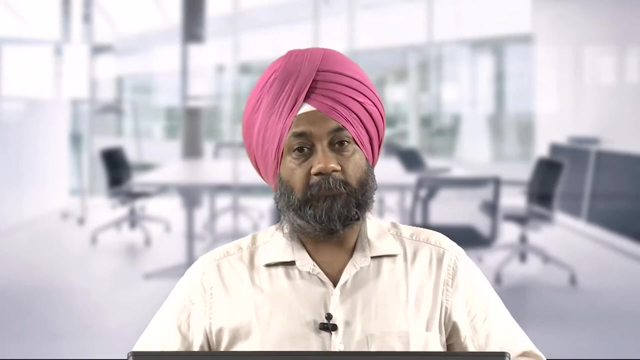 a product designer must know, Every product designer must have a basic idea about the materials, otherwise how the designer will be able to specify that this particular material can be used for this specific application? Again, I am taking an example. Okay, I am taking the example of a chair. 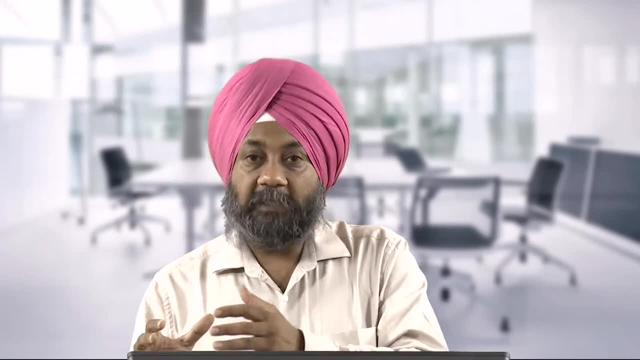 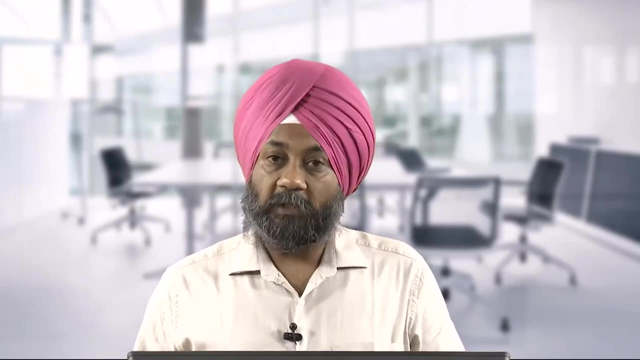 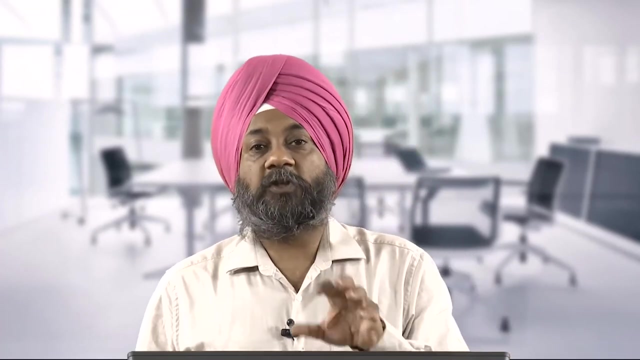 In chair. if you see, a chair can be made with metal, it can be made with wood, it can be made with plastic. Now we have different types of chairs now, depending upon the specific application, the product designer has to find out, has to suggest that which material must be used for this particular 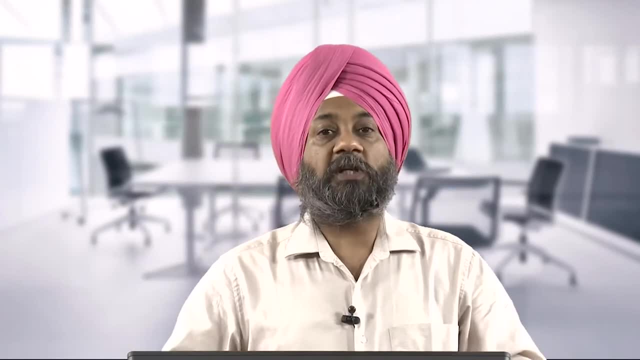 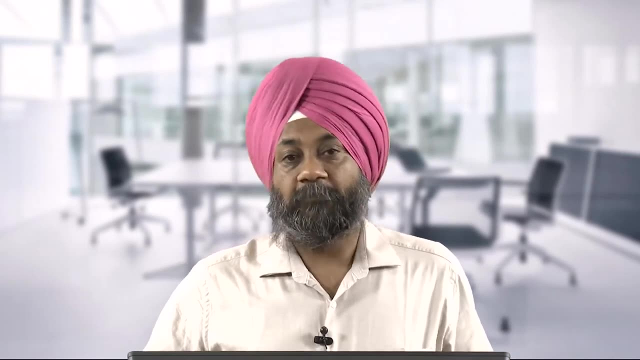 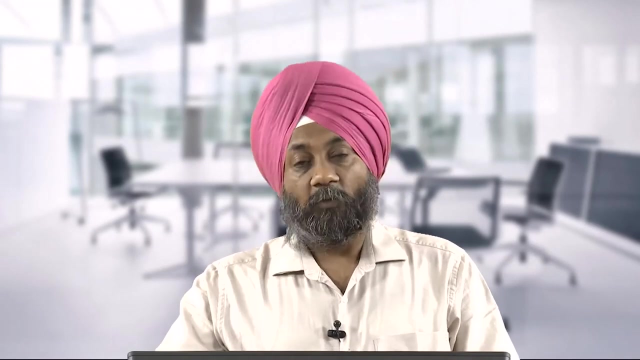 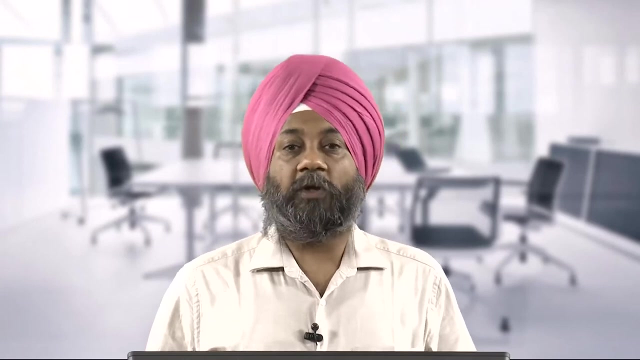 type of a chair. So the properties of the engineering materials must be known to the product designer prior to finishing, or prior to finalizing his or her product design. So we will try to revise what are the various mechanical, physical, chemical properties, as well as the thermal properties which are important from the product design point of 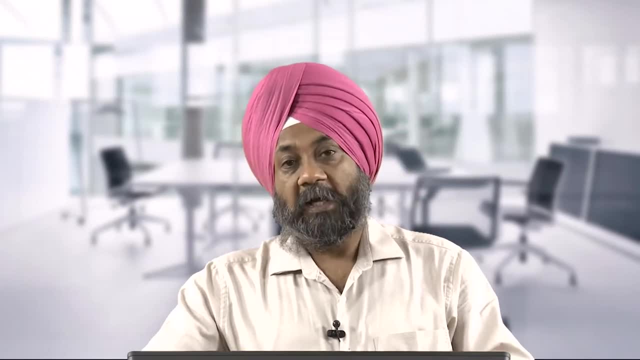 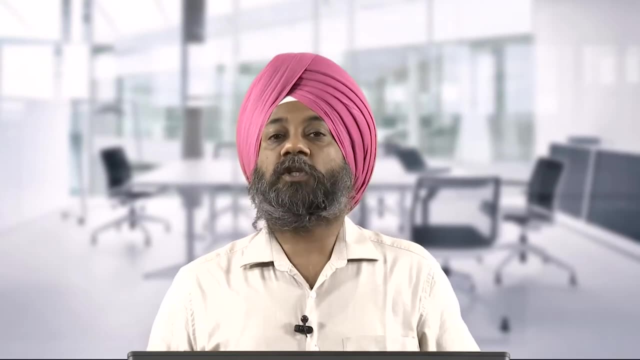 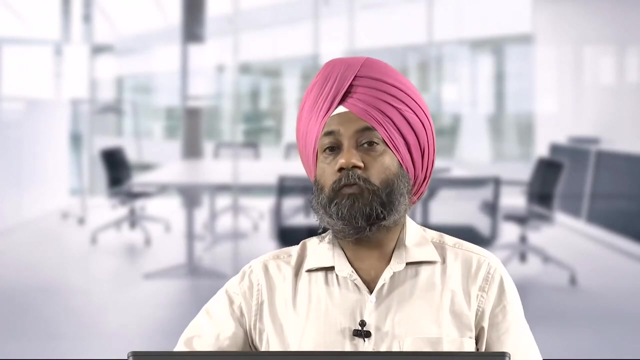 view. So whenever we are designing a product, we must have a look at these properties from the material suggestion point of view or from the material choice point of view, because whenever we finalize a product, we have to see that which material is going to be used for designing. 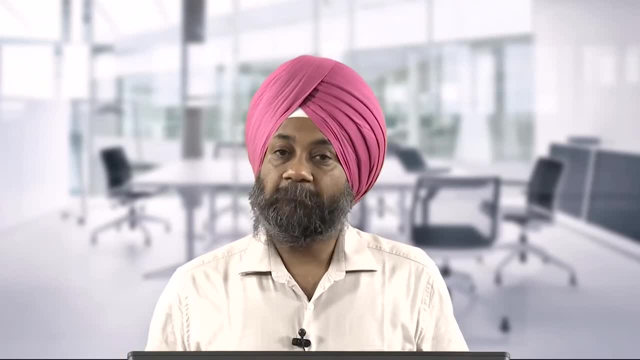 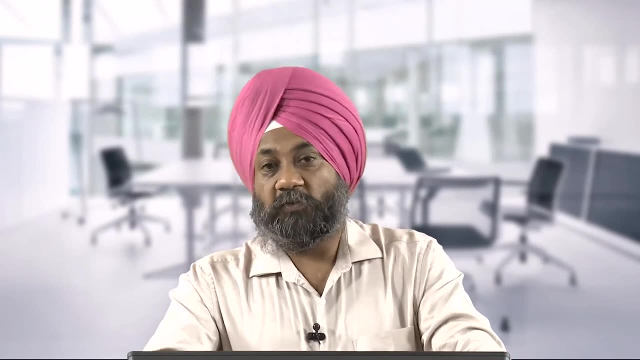 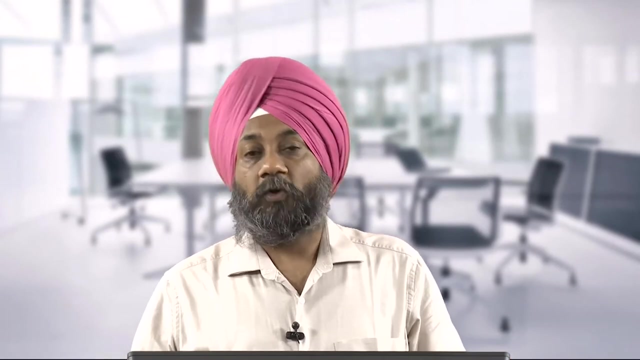 or for after designing, for fabrication of this product. One example that I usually take in the class is the example of a toothbrush. In toothbrush we see what are the basic requirements. it must be light in weight. it must be cost effective. it must not be too costly. 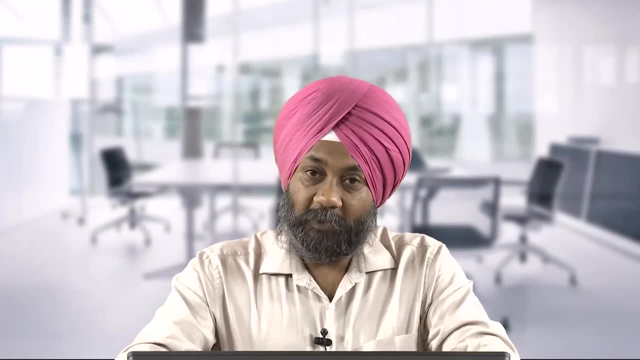 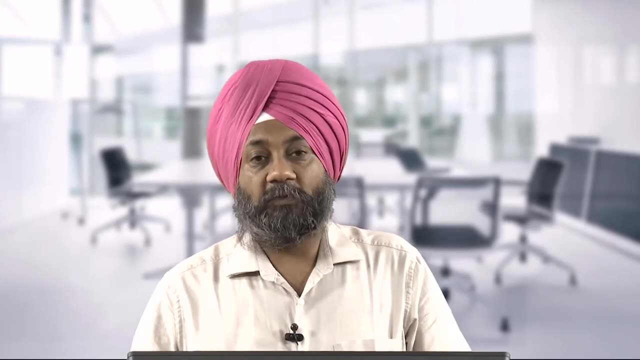 Then the bristles have to be light. They have to be light- Light on the gums, or they have to be soft on the gums or they have to be harsh on the gums. Most of the time we see bleeding from the gums if you brush your teeth too vigorously. 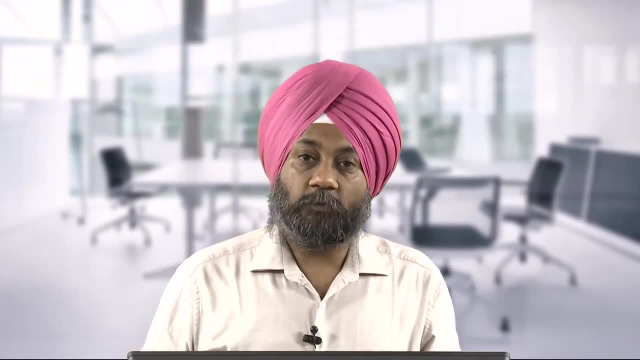 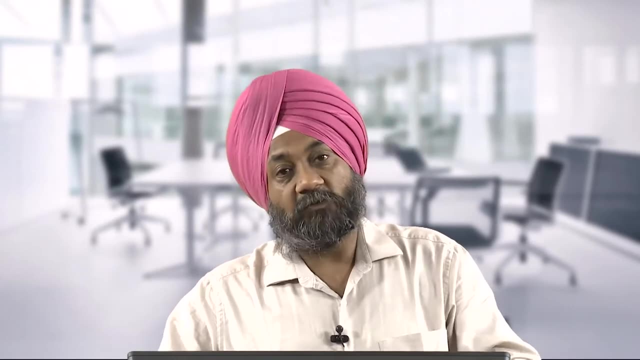 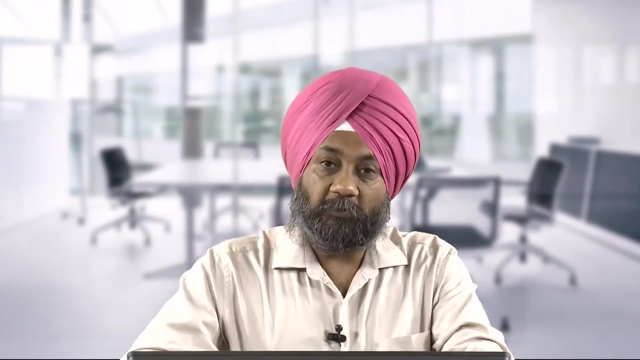 So we have to ensure that the material of the bristles must be soft on our gums. So we cannot use a metallic bristles in case of brushing of our teeth, whereas we can use the metallic bristles for some other application where we want to do hard rubbing on any surface. 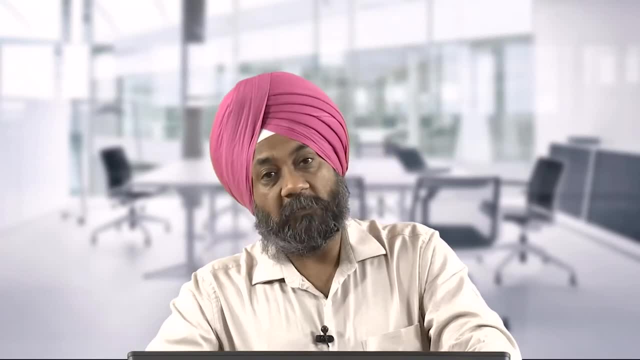 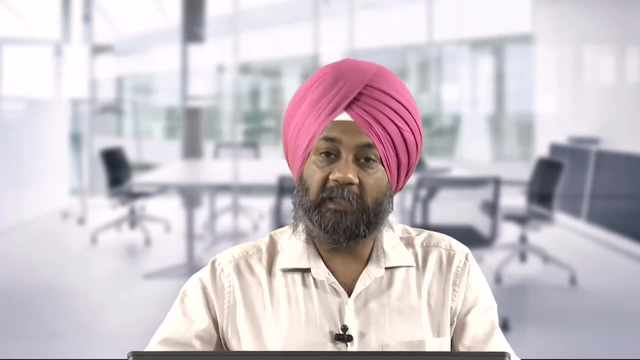 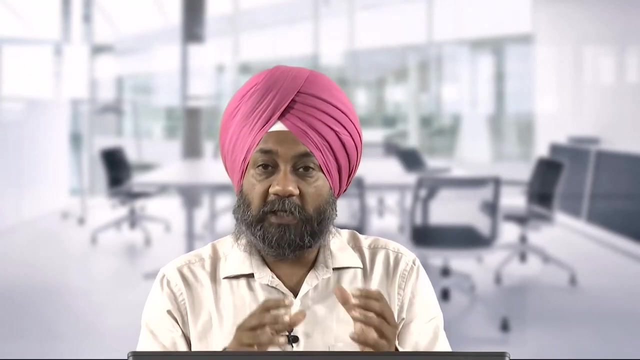 or we want to do cleaning of some very hard surface. There we may go for metallic bristles, but in case of toothbrush we will definitely suggest soft bristles only, and then the material that we select must be soft on our gums. So this is just one example of selection of a material for a specific product and how 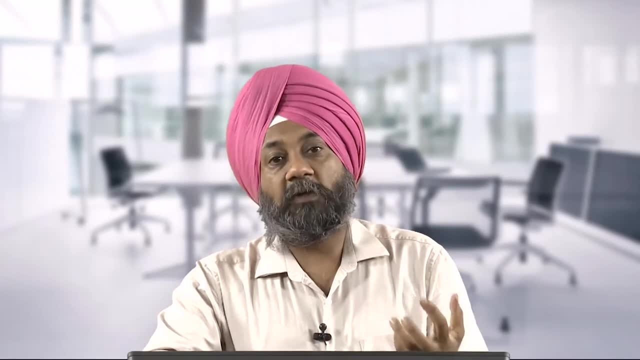 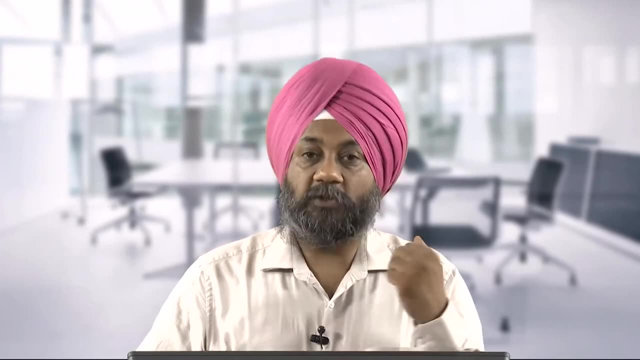 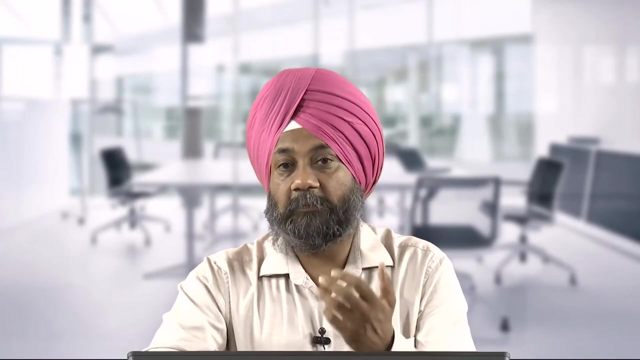 we will be able to suggest the materials for products if we have complete information about the materials, The types of materials, The types of materials available, as well as the properties of the materials. and then we must also know that how to select the materials, What can be the selection criteria based on which we can select the material for a specific 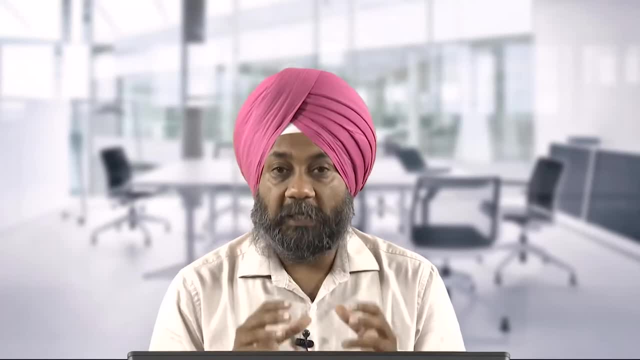 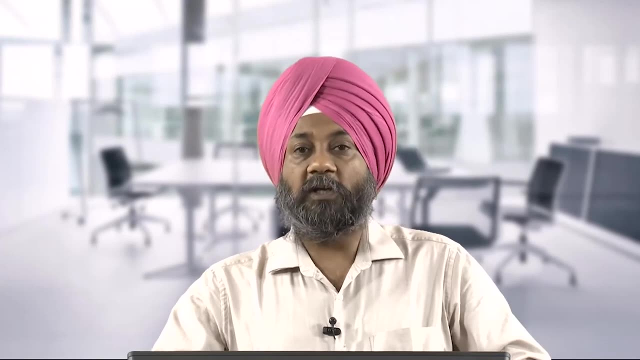 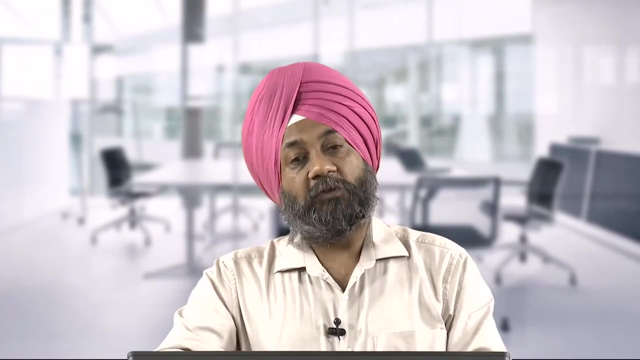 application, and that is the objective or the aim, or we can say the goal, of this particular discussion that we are having during this week. That is the second week of our course on manufacturing guidelines for product design, So let us start our discussion. Let us start our discussion with the properties of materials. 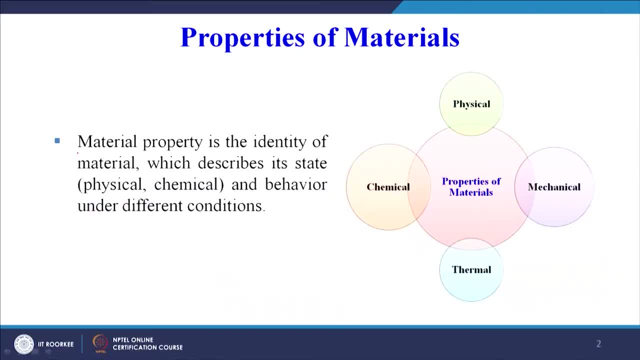 Now, what are the properties of materials? You can see, a material property is the identity of the material. So identity, it will identify the material. Now, how it will be identified? It will be identified based on the physical, based on the chemical as well as based on. 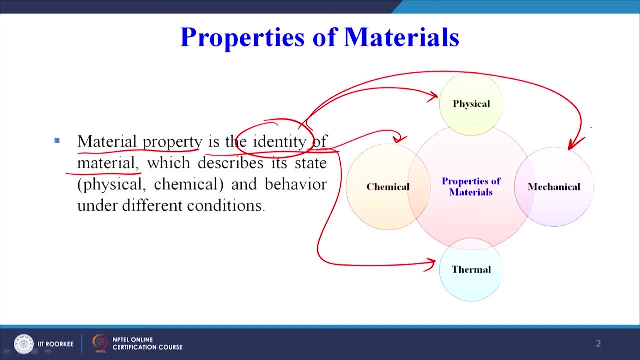 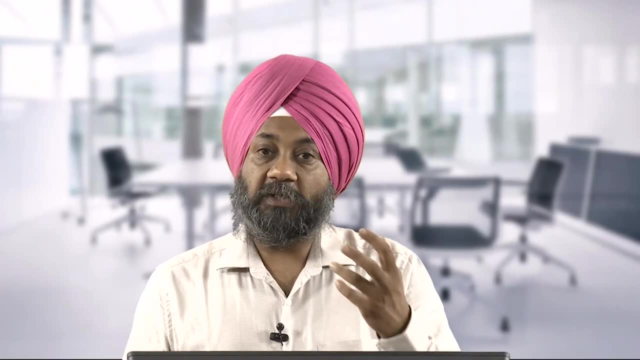 the thermal and the mechanical properties of the material. So the material property is the identity, Identity of the material which describes its state, physical and chemical state- and the behaviour under different conditions. So the property basically will define the behaviour of a material under different conditions. 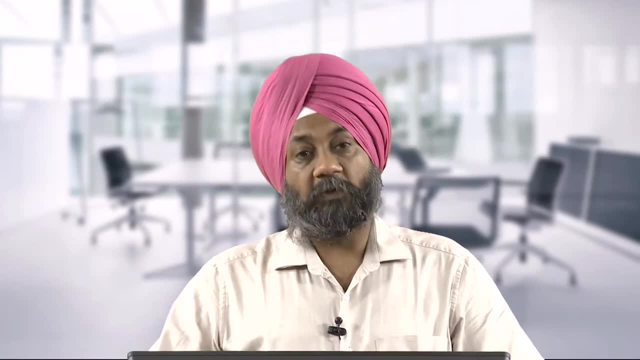 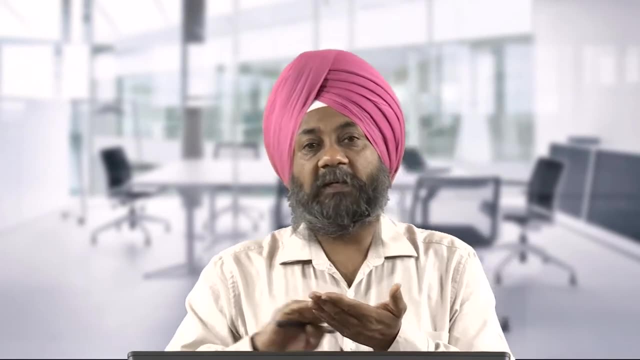 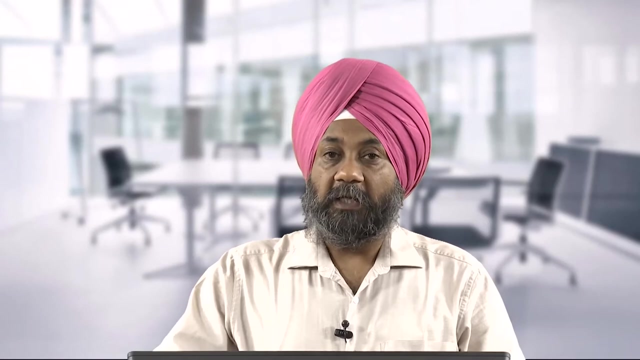 How it is going to behave when it is subjected to different types of conditions. For example, if we have a surface and we rub on the surface, we will try to see that what is one of the properties That may come to our mind may be the hardness of the material. 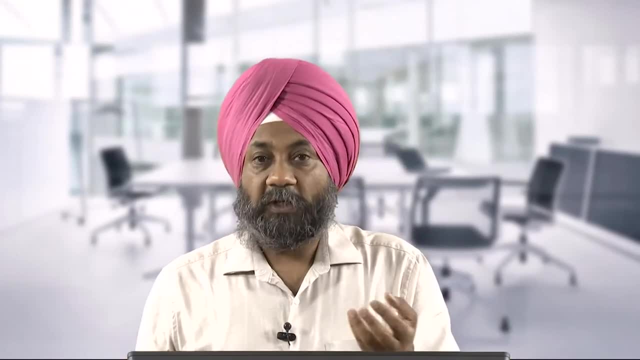 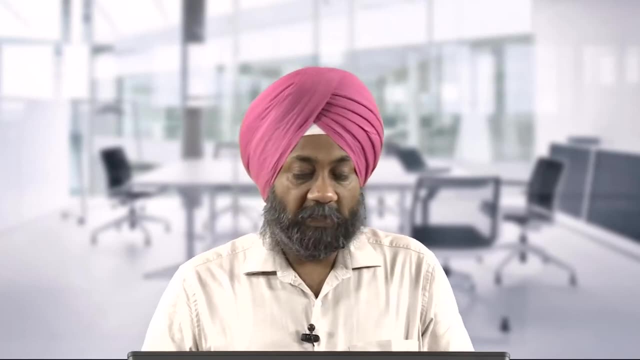 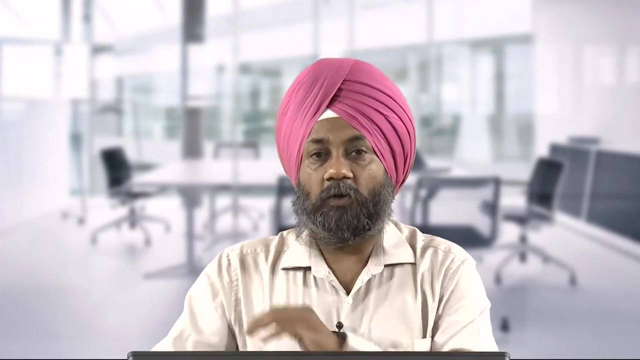 If it is hard, it will wear out less, If it is soft, it will wear out quickly. So then we have to see that how the material will behave under different types of conditions. So that is going to and that will be dictated by the various properties of the material. 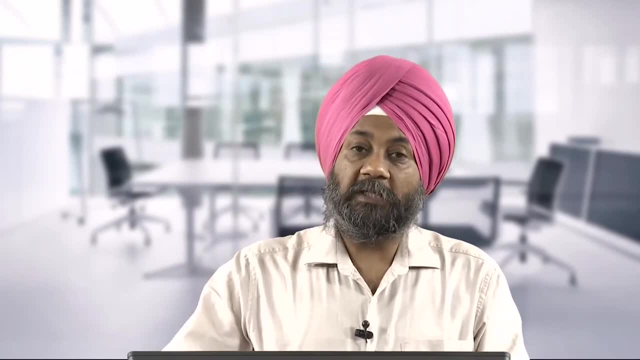 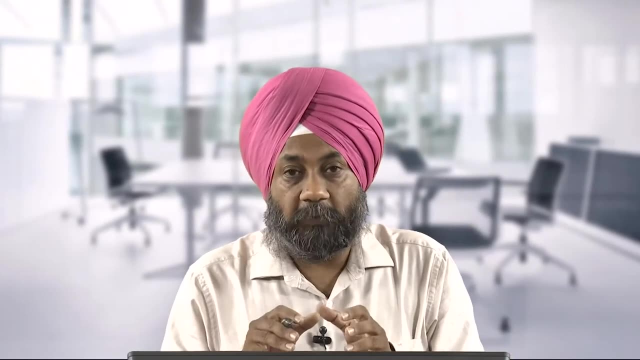 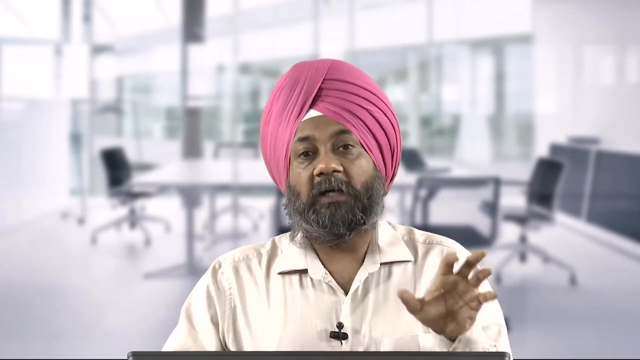 So steel may have a different wear resistant properties, whereas plastics may have a different wear resistant properties. And from application point of view, this example, if we can talk about the floor, So many people are walking on the floor, So we must know that how this flooring is going to behave when may be hundreds of people. 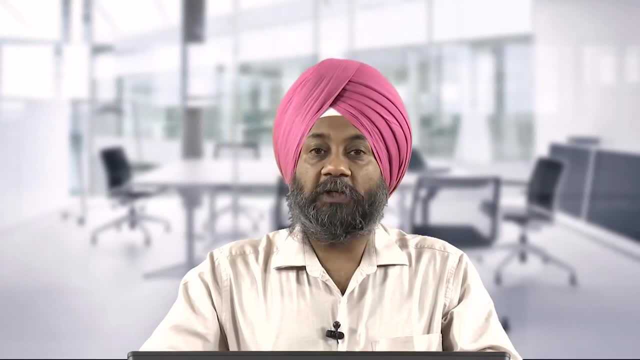 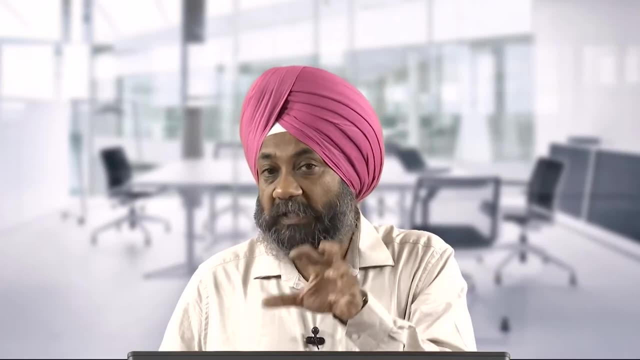 are going to walk on this floor. It must not wear out, It must not decolor, It must not be. chipping of material may not take place from the floor. So how we will decide that which material must be selected for our floor. 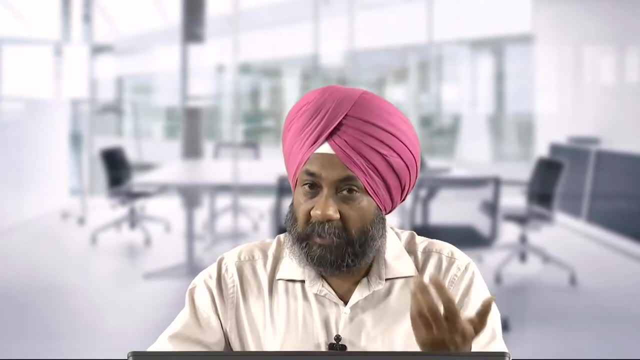 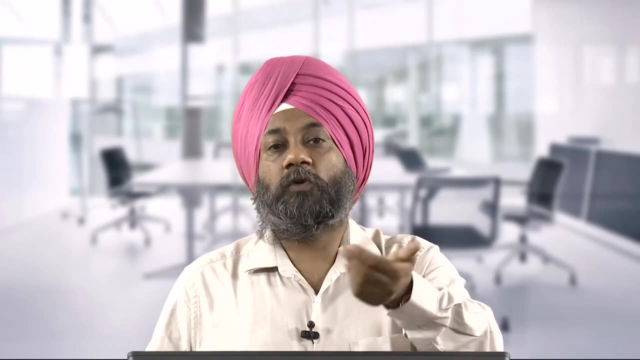 It must not wear out, It must be tiles, It must be a carpet, or what type of flooring we must provide when so many number of people or X number of people are going to walk on this floor on daily basis, on weekly basis and on yearly basis? 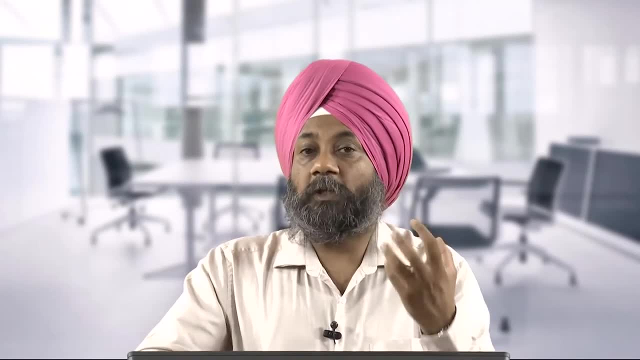 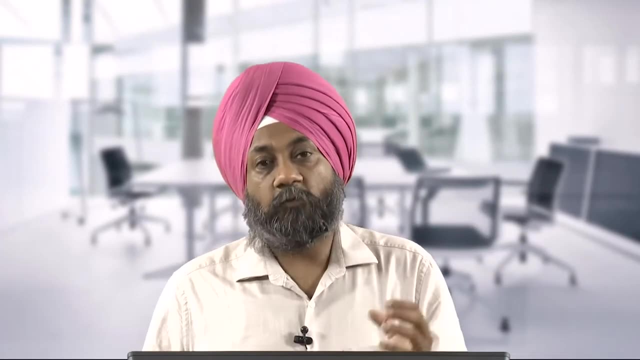 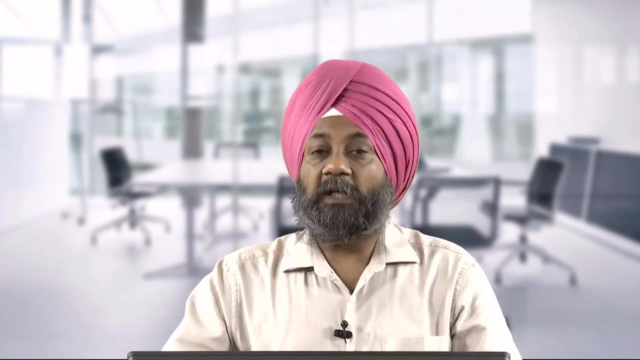 So that selection of material will depend upon the properties of the material that, yes, this material possesses these specific properties and therefore it can be used for this specific application, for making the floor. So that is why the importance of material properties cannot be ignored from the product. 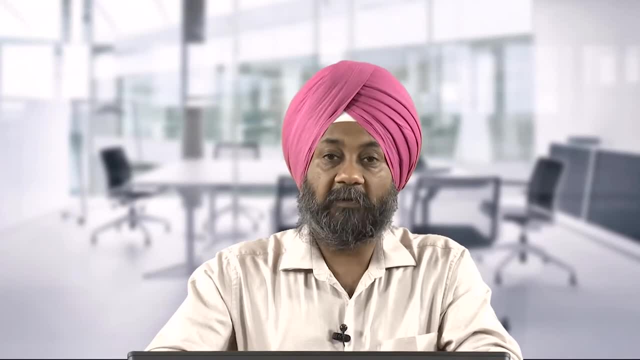 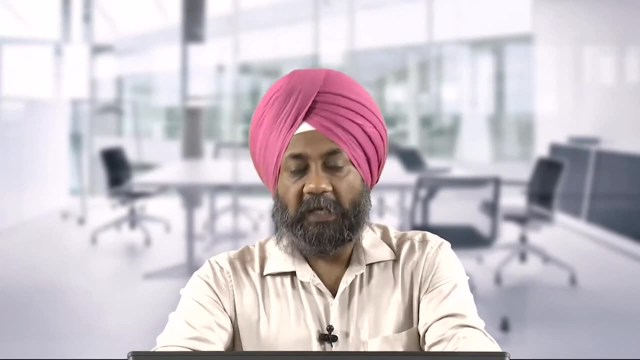 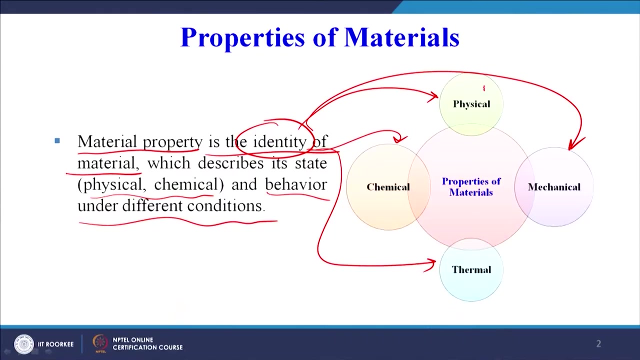 design point of view, And every product designer must have little information, or we can say a basic information, about the material properties and the focus primarily has to be on these 4 properties that we have listed here. So first one can be the physical properties. 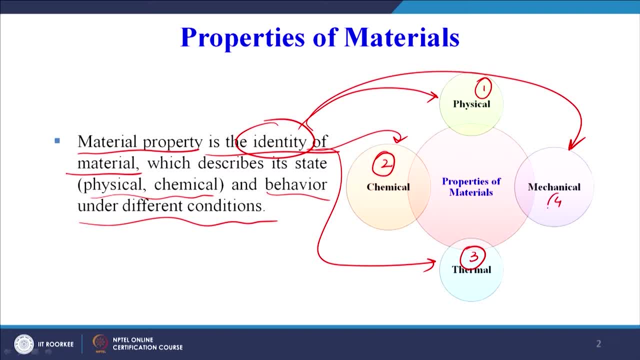 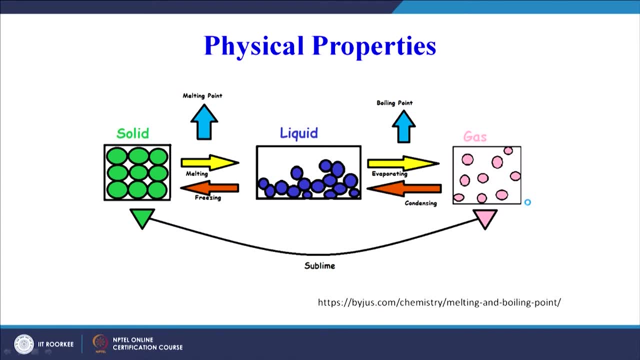 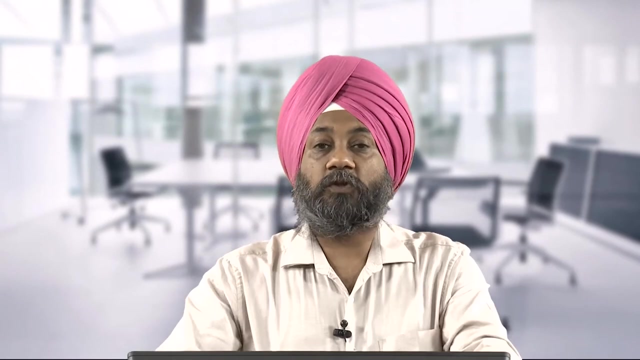 The chemical properties, The thermal properties and the mechanical properties. So we will see each one of these in today's session. Now, what are the physical properties? The physical properties are, maybe it is mentioned here- the melting point, the boiling point of the material, we must know, and the phase change, maybe sublimation characteristics of 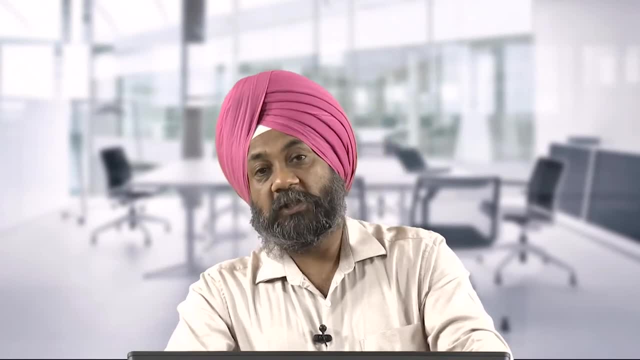 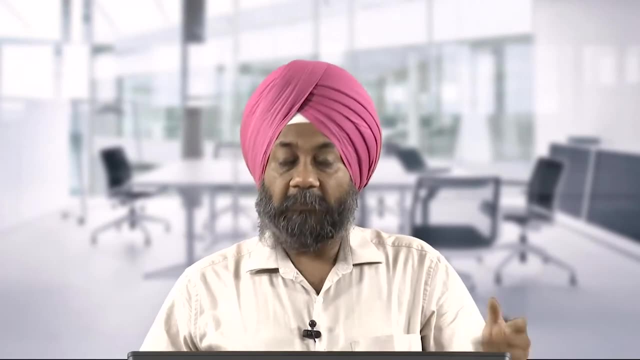 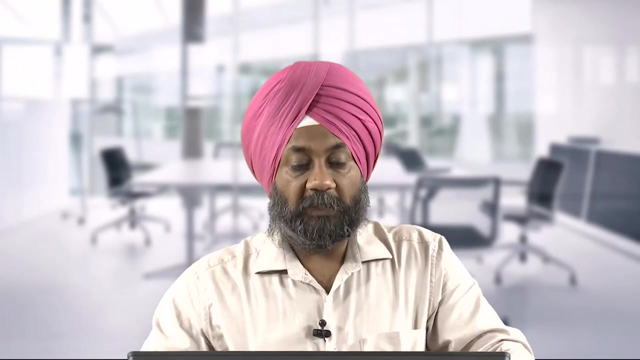 the material must be known to us how it will change from solid to liquid, at what temperature That transformation will change take place from liquid to gas. at what temperature this is going to take place? what is the boiling point of the material? what is the freezing point of the material? what is the melting point of the material? all these properties? 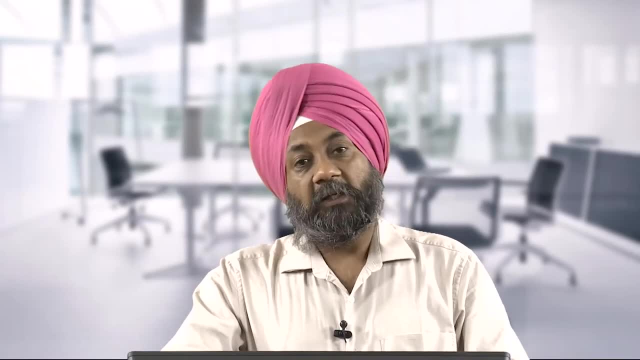 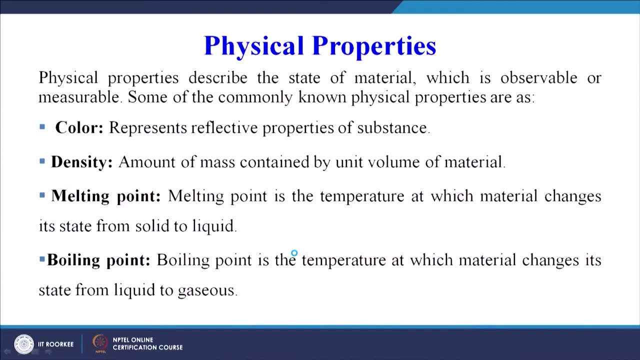 must be known to the product designer when he or she is designing the product. So what are the physical properties? Now, physical properties describe the state of material. So these describe the state of material Which is observable or measurable. So these are the 2 key characteristics: observable and measurable. 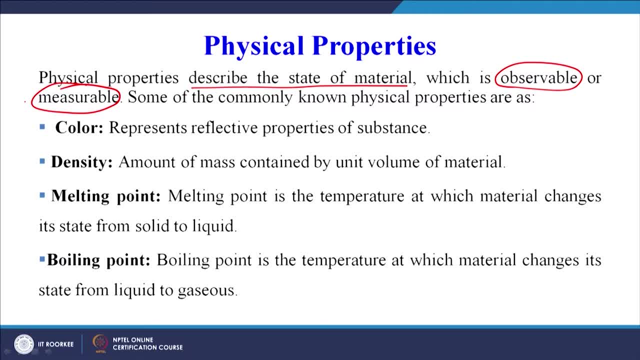 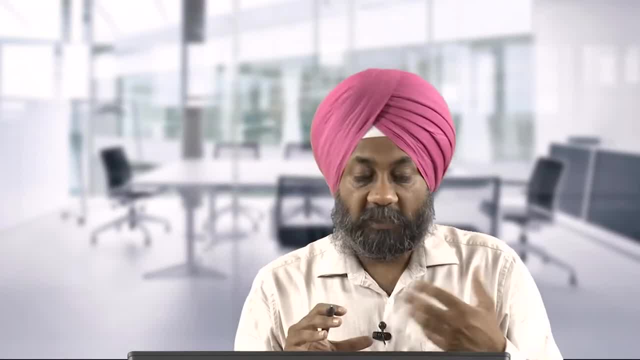 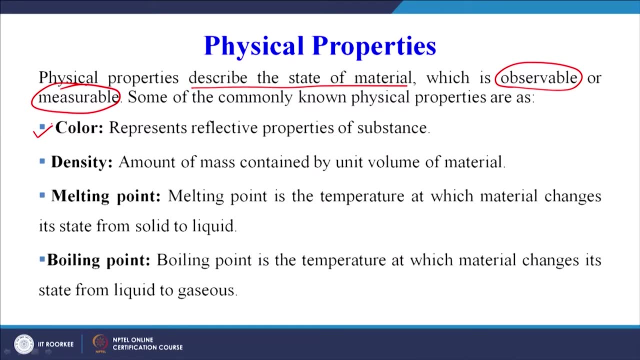 Some of the commonly used physical properties are. we can go one by one. So we have to see that the properties which we call as the physical properties are observable as well as measurable, So we can see. color is one property, represents the reflective properties of a substance. 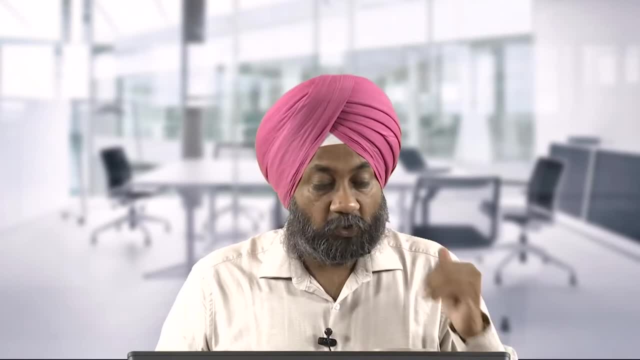 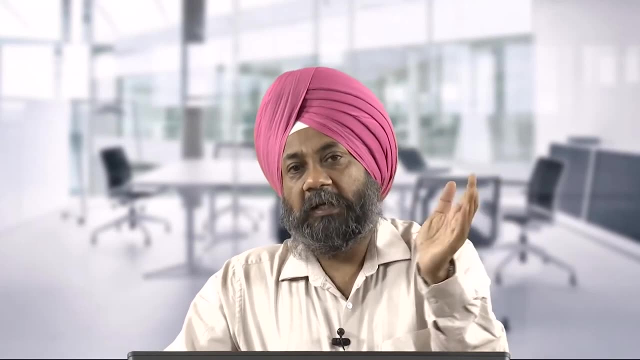 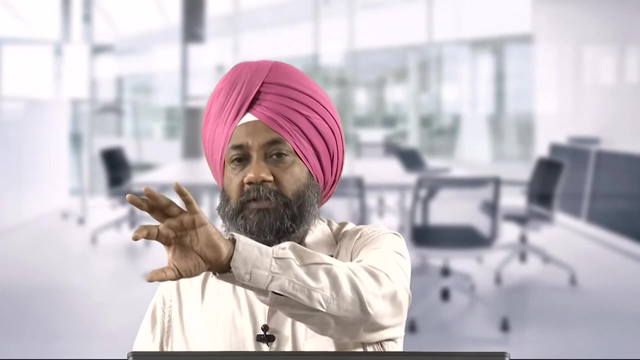 So we can easily grade the material. So we can easily grade the material Based on the color and if you see some of the advertisements, they show the different color, but before this is the color, after this is the color. So that is measurable: that before the treatment this is the color, after the treatment, this 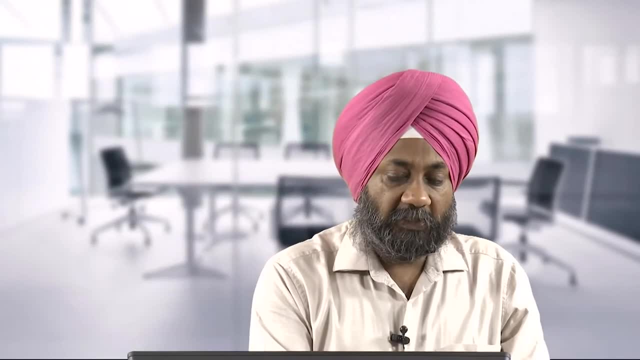 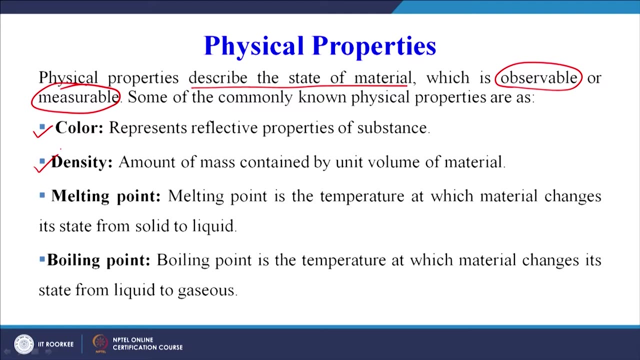 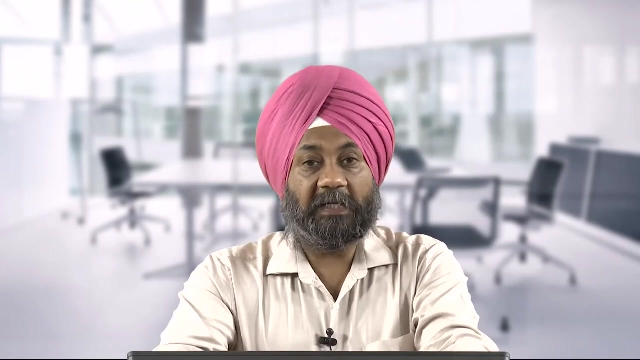 is the color. So that is one physical property. then density: amount of mass contained by unit volume of material. So this is another physical property which we must know and this is very, very important when we design the product, When we are designing the product and we want it to be very, very light in weight. 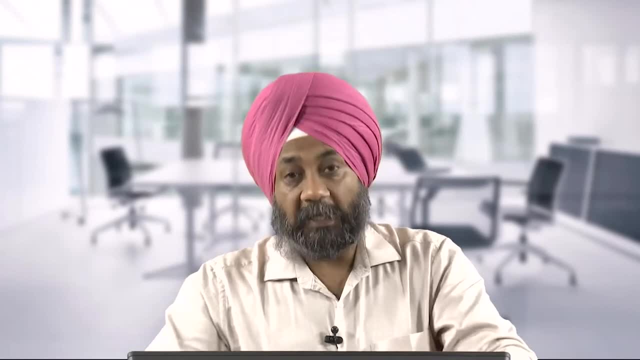 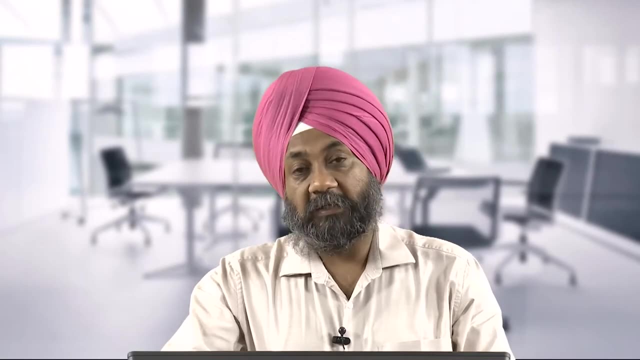 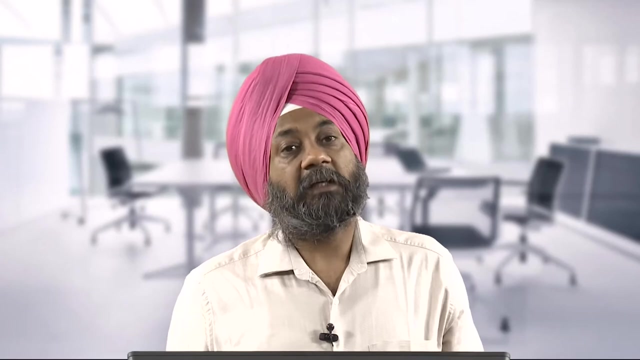 So we have to understand that which material can provide us this light weight product. So we will definitely compare the densities of the different materials and try to see that wherever it is possible for us to save some weight, we will select the material which will have density accordingly. 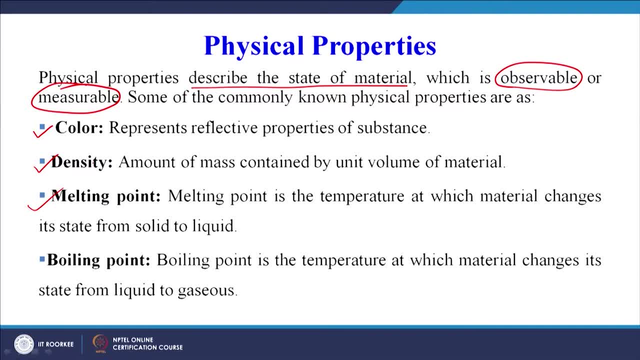 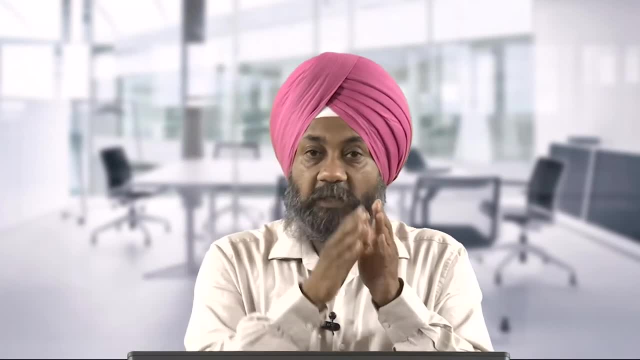 Similarly, the melting point of the material. the melting point is the temperate temperature at which changes its state from solid to liquid. So that melting point, if you remember, we have seen in the first session when we were discussing the manufacturing processes. we have seen one graph on y axis. we had the melting temperature. 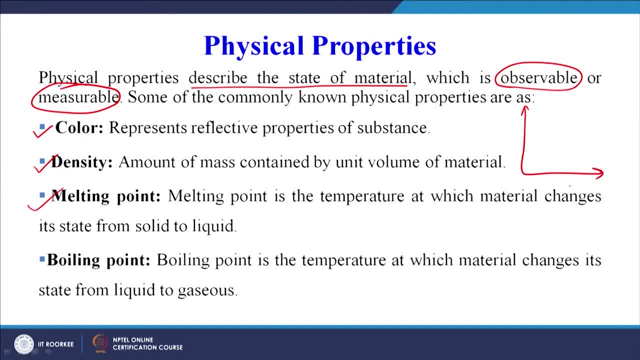 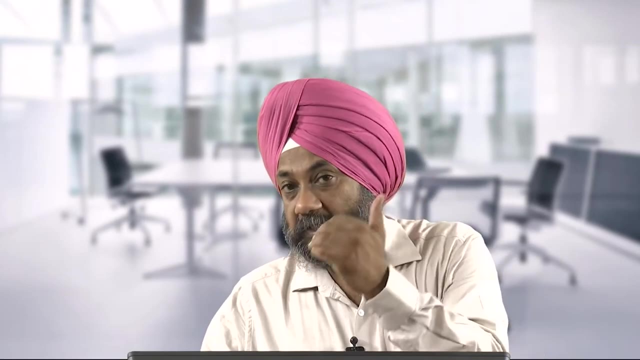 If you remember, for the various manufacturing processes we have seen this type of graph: on y axis we had the melting temperature or the melting point, and on x axis we had the volume of production and then we have put different processes there. So melting point is an important parameter from the material selection point of view. 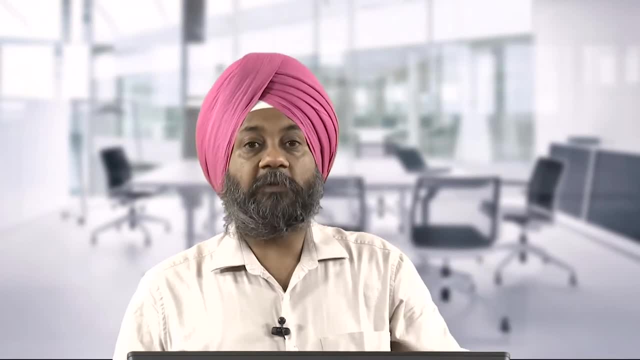 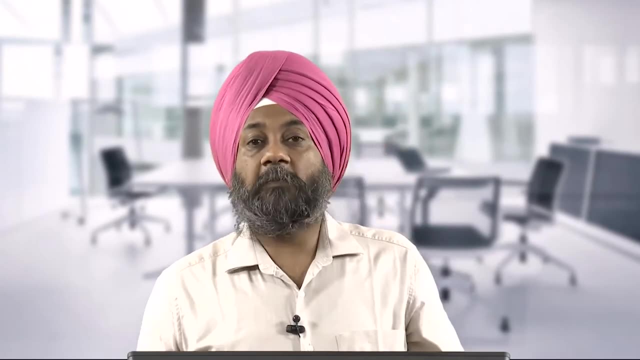 and subsequently it will affect that which process can be used for making the product. So if we are selecting a material which is having a very high melting point, we may not be able to make it by casting process, So therefore we may have to suggest a different process. 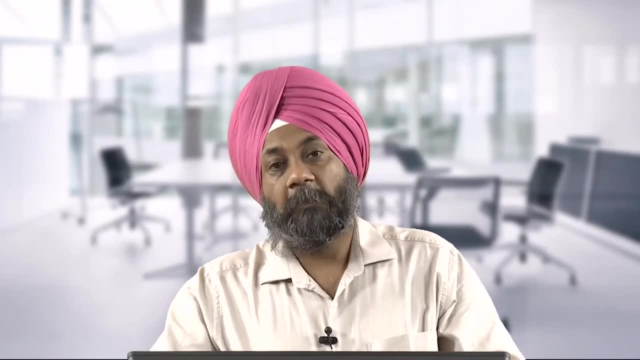 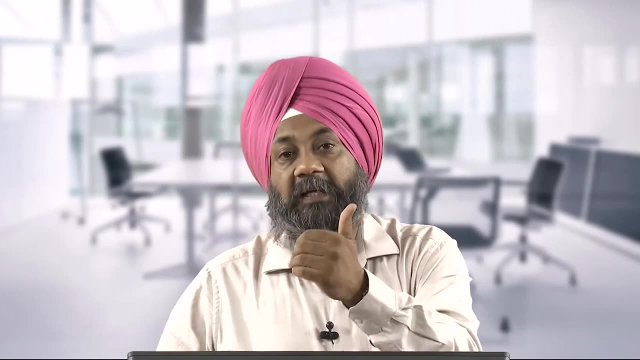 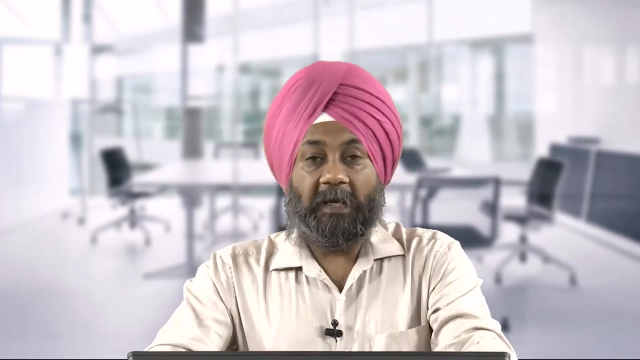 Where the melting point is not going to play an important role. So, but the melting point high material that we are selecting for a product may have certain special characteristics. thereby we are suggesting that high melting point material must be used for this specific application, and if we are suggesting a material for a particular application, 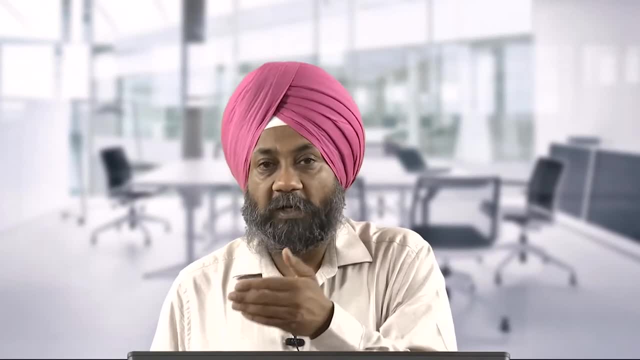 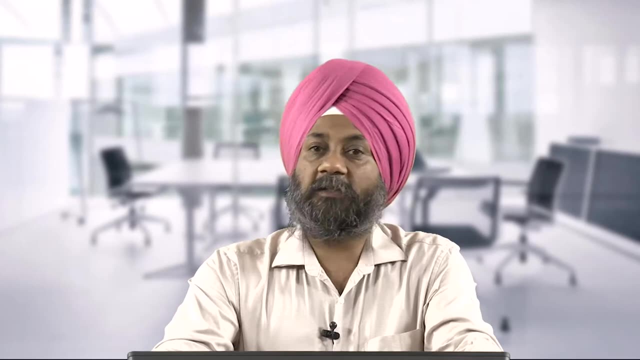 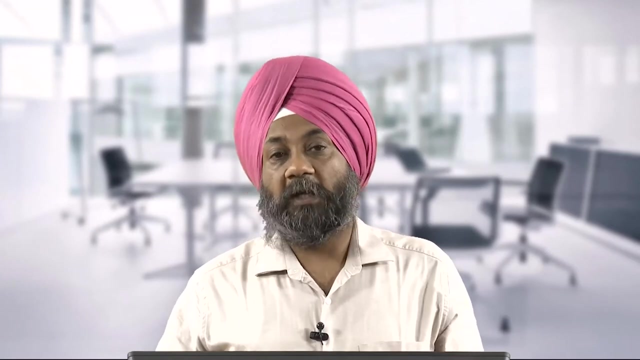 where the melting point is low, we will suggest: since the melting point is low, we can use casting process for making this product, Because easily the furnace will be Able to convert the raw material from solid to liquid form. So therefore, this knowledge of these properties is going to be helpful for the product designer. 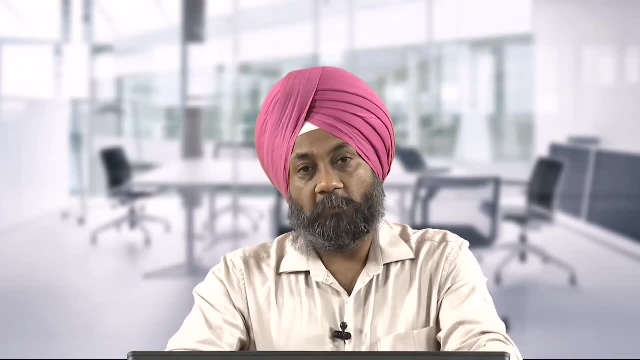 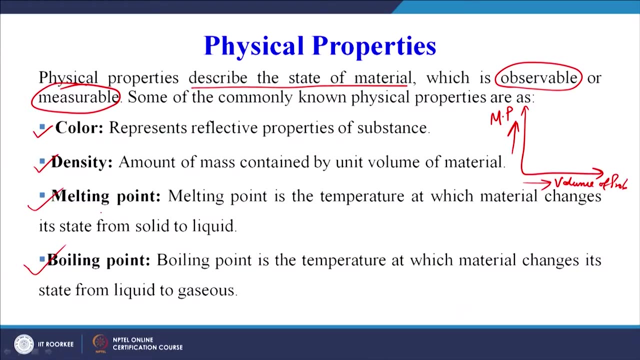 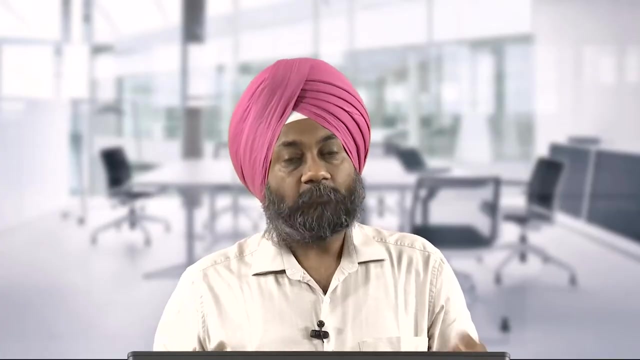 for appropriate selection of the material for the product being designed. Similarly, the boiling point also is very, very important. So boiling point is the temperature at which material changes its state from liquid to gas, as we have seen in the previous slide. So when we are talking about 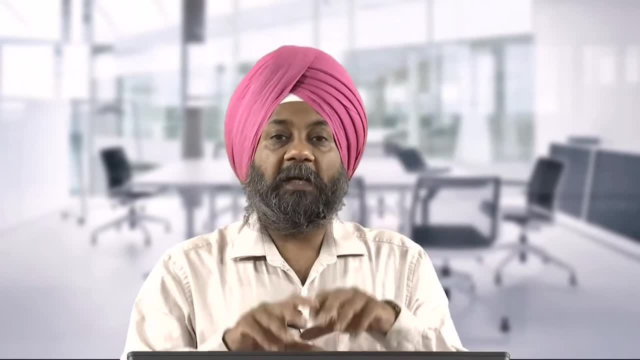 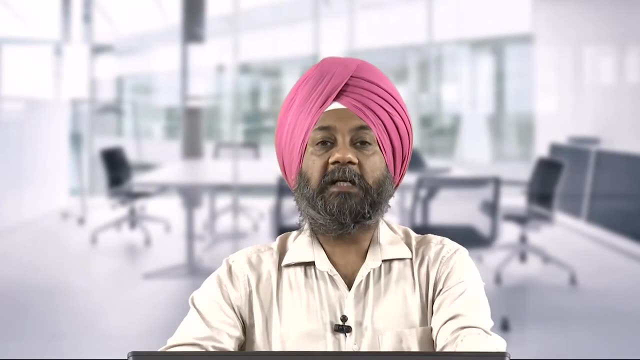 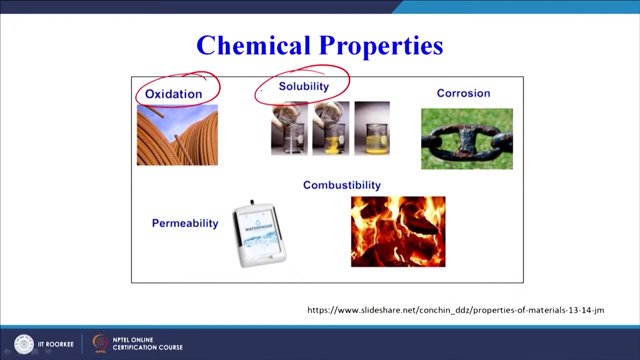 The materials. properties of the materials. we have 4 broad categories. The first one are the physical properties. then we will go to the chemical properties and on your screen you can see this is the property of oxidation, solubility, corrosion, permeability, combustibility. So these are just, we can say, representative chemical properties. there can be a extended 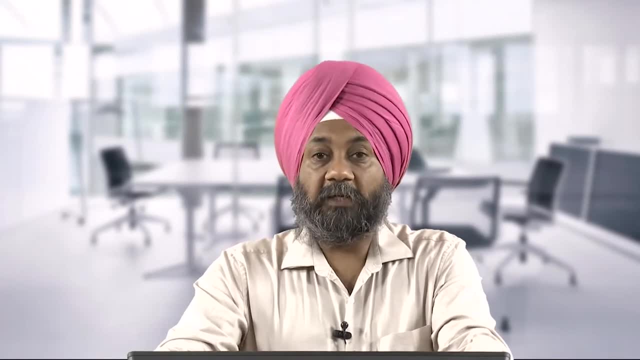 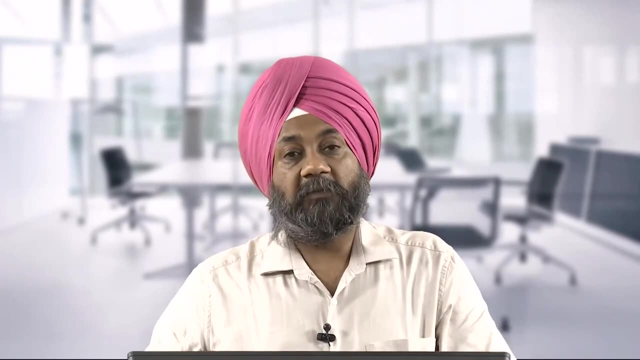 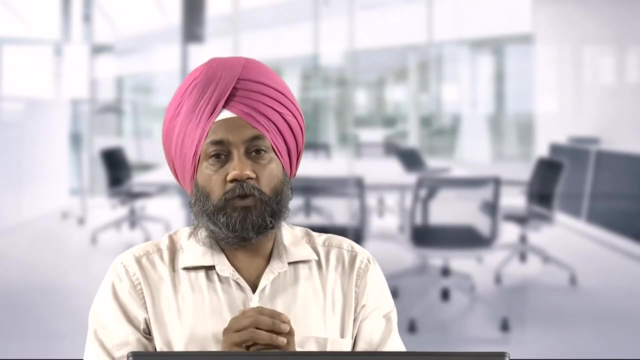 list of chemical properties which must be taken into account before finalizing a material for a particular product. and these are a representative list only. So we have seen, suppose we have to understand. we want to mix 2 different solvents together for a particular application. we must know the property of solubility of each one of them. 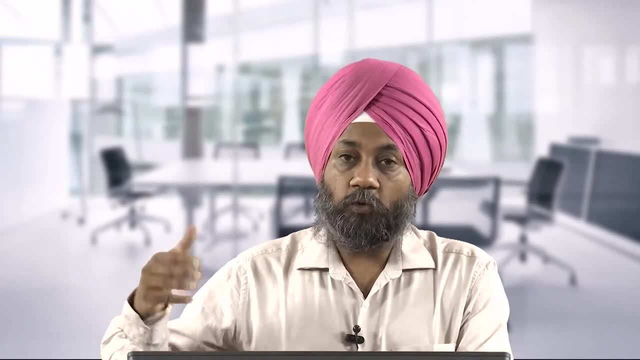 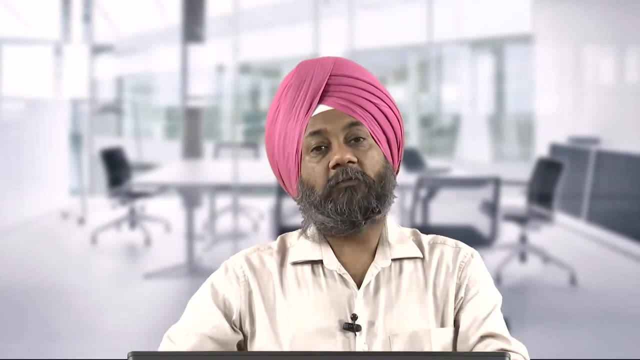 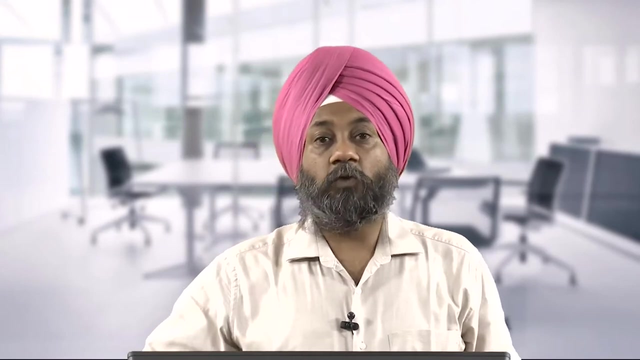 Similarly, if we are suggesting a material which has to be outdoor or it has to be underwater For All of its life or throughout its life, it is a underwater installation. we have to be very, very sure about the corrosion properties. Sometimes we try to improve the corrosion behaviour of any substrate by putting lot. 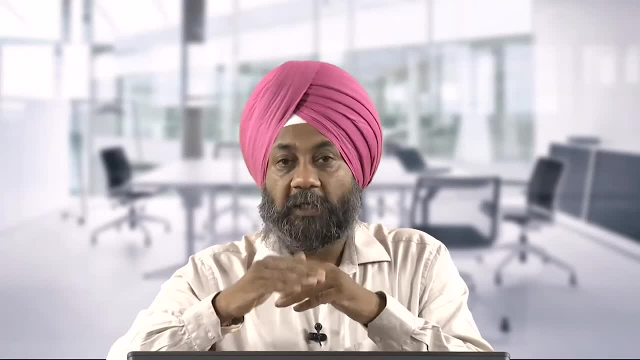 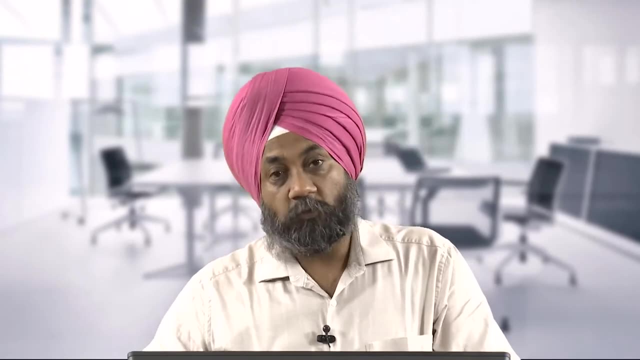 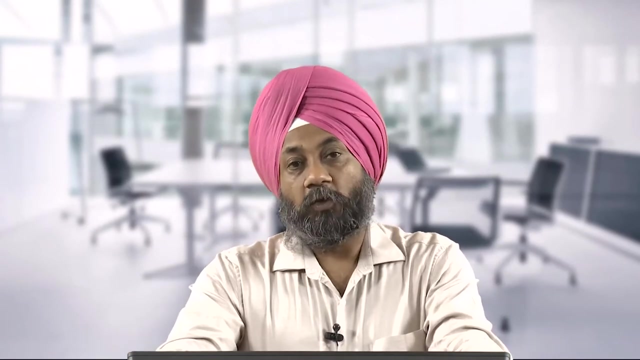 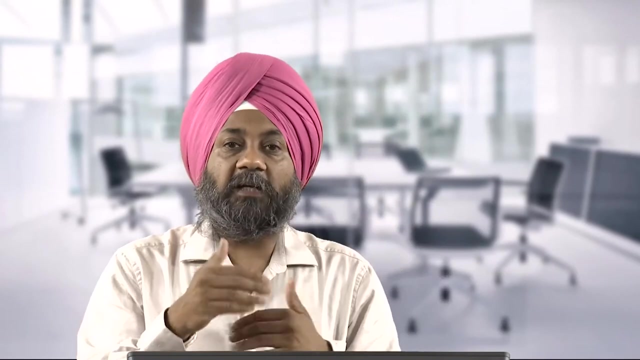 of coatings on the substrate. So the coating improves the corrosion behaviour of the material. it reduces the corrosion rate. So this type of coatings can be given on the substrate To avoid the corrosion or the problem caused by corrosion. So this must be known when we are suggesting a material which has to be constantly in contact. 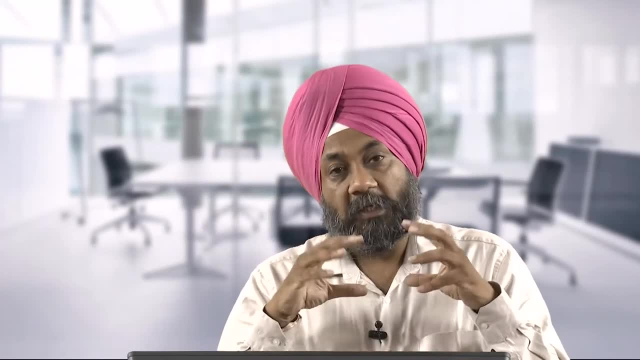 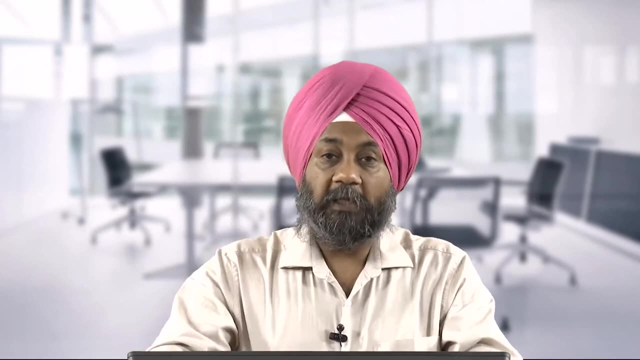 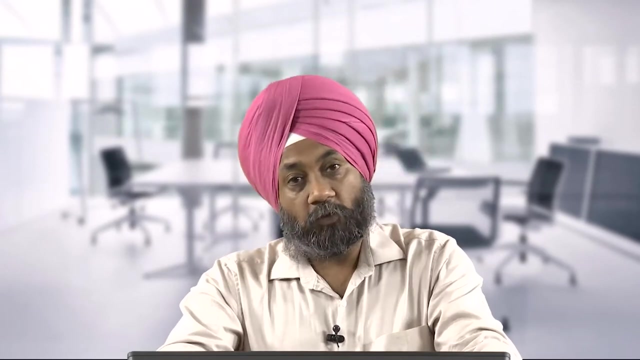 with water or constantly in contact with some chemical regions. We need to understand that how it the life of the product will be affected, whether the corrosion will take place or not, or what is the corrosive behaviour of this material, and therefore we need to understand these properties from the product design point of view. 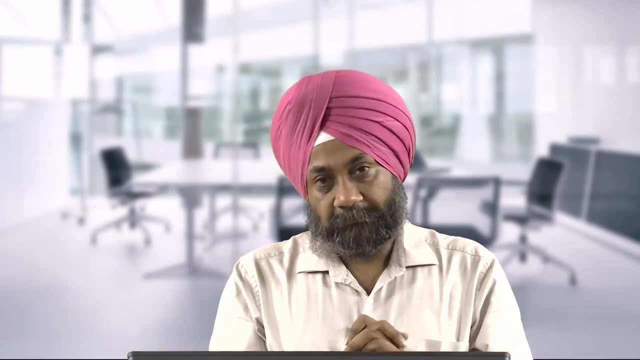 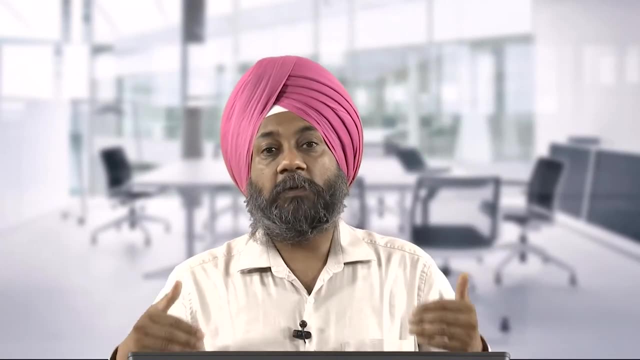 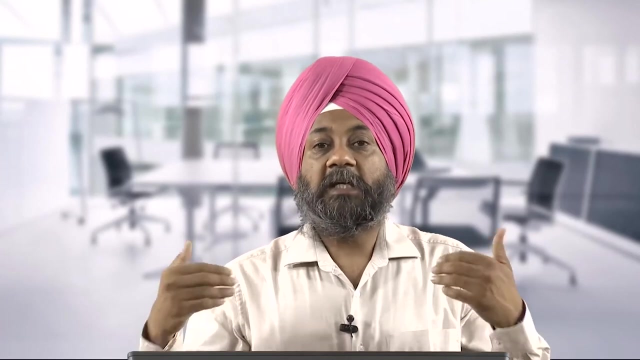 Because many times from the suppose we make a product, the product is put into service and then during the service, we have to suggest that this has to be maintained, this has to be serviced after so many hours or so many weeks or so many months or so many years. 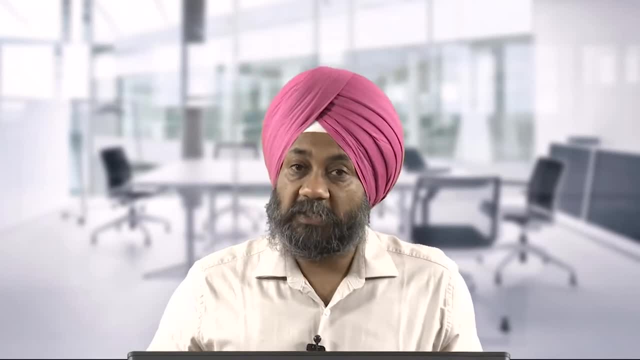 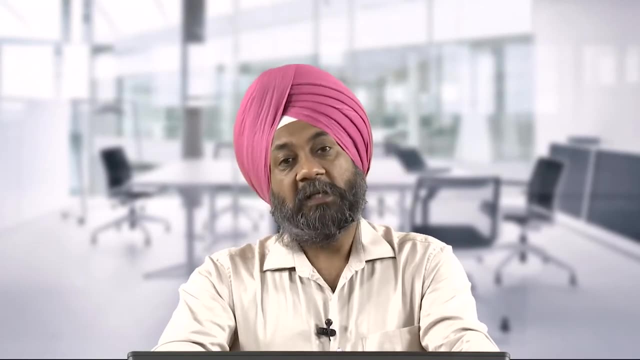 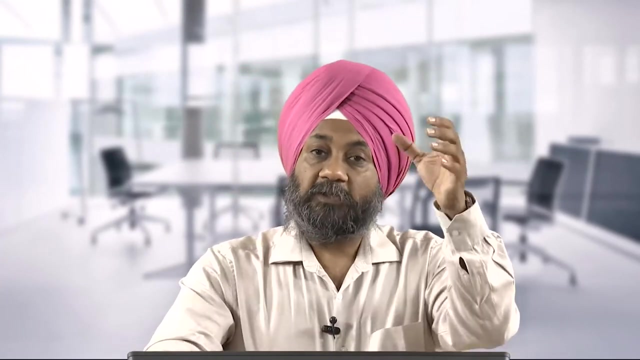 So regular maintenance has also to be suggested. Many times we have maintenance in terms of you have to paint the surface every year or every 18 months. So why that painting is required? because sometimes the corrosion may start at the surface of the material. So for that particular material, when we are suggesting it, for a particular product or 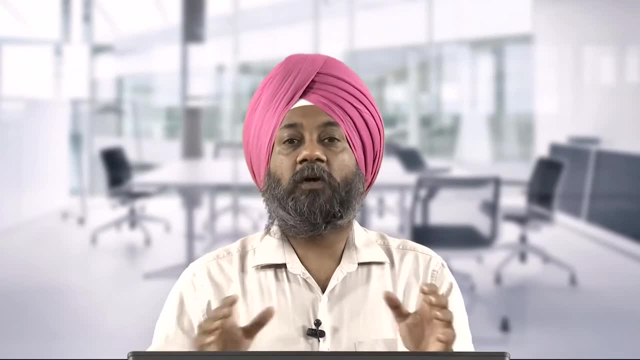 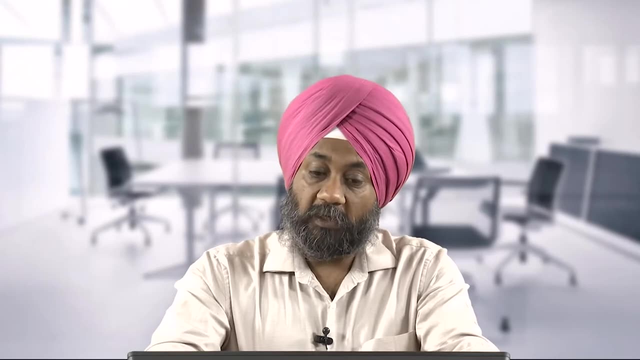 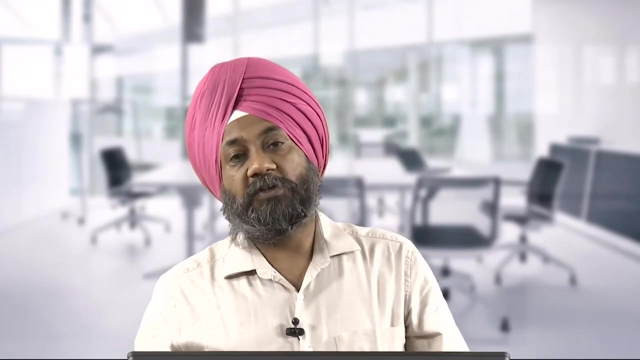 a structure or a bridge, We must know that how it is going to behave under the various service conditions and therefore we must know the corrosion behaviour For each properties. I am taking one example. in the last I have taken example for physical properties from for the melting point. I have tried to explain the importance of melting. 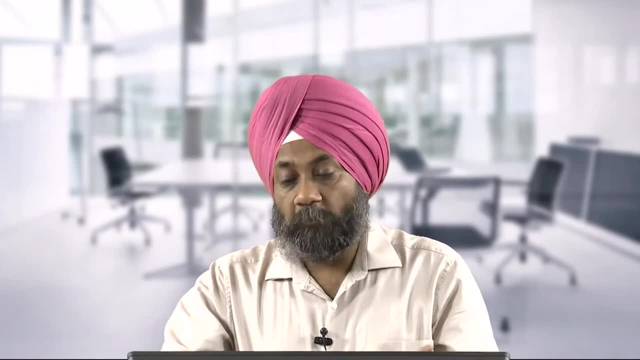 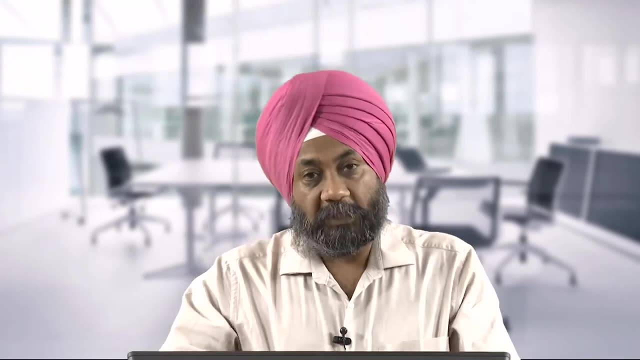 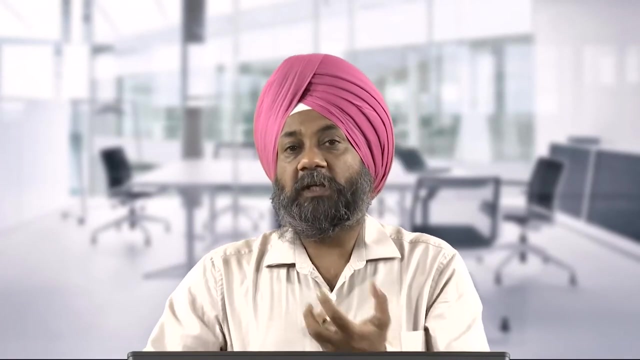 point. In chemical properties, I am trying to explain the importance of corrosion. similarly, the combustibility, solubility, oxidation, permeability, All these properties. we can take example of each one of these and try to understand that. what is their importance? What is their importance from the product design point of view? 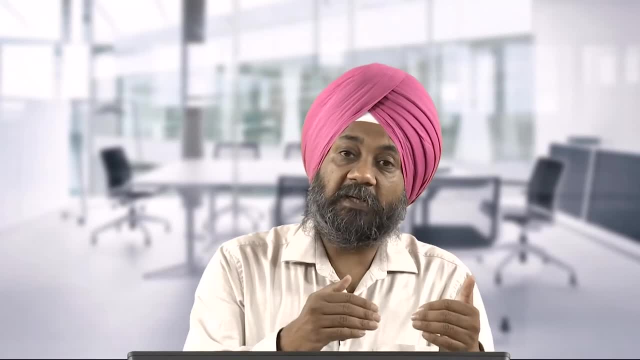 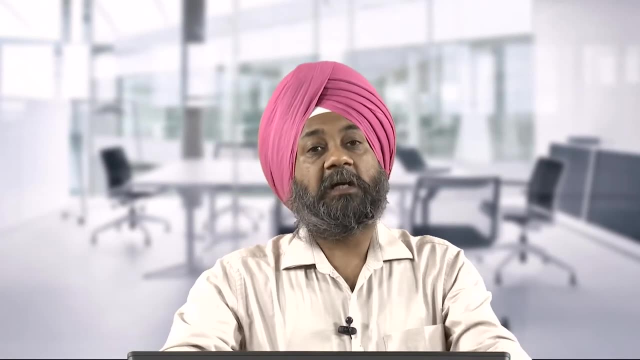 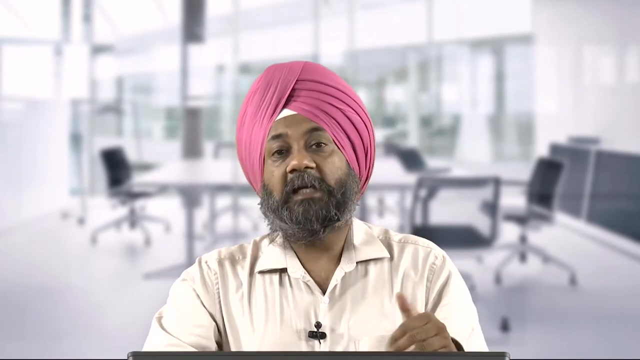 So from the combustibility we can say that wherever we are suggesting polymers. So we have to have clear idea about the flame retardant behaviour of these materials And if we know that there are chances of fire, we must add fire retardant regions or fire. 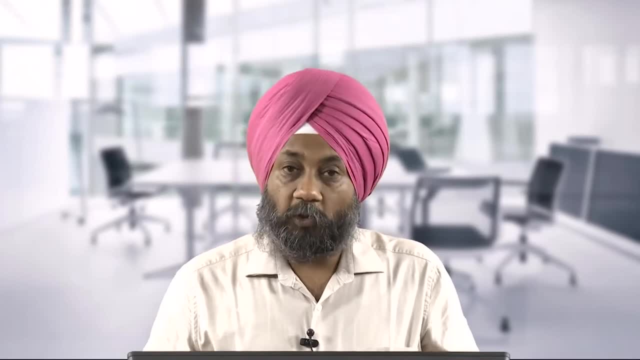 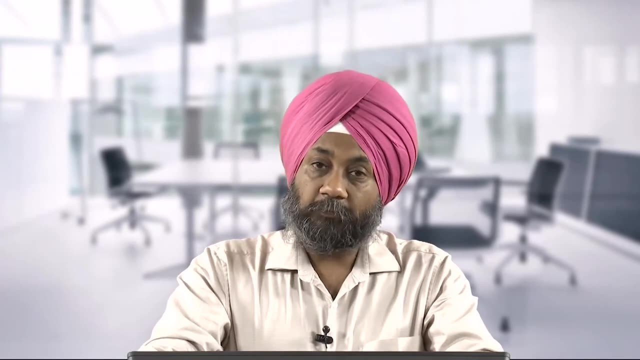 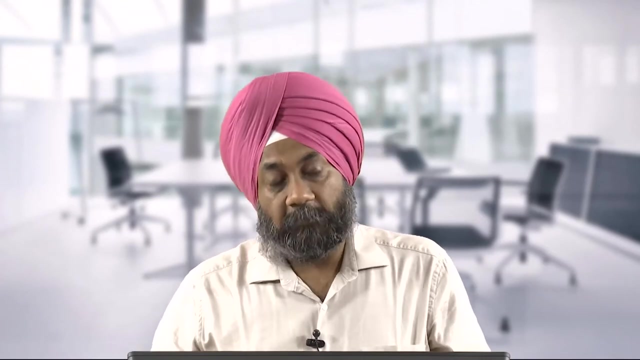 retardant additives into our polymer products. We must know that what is the combustibility or flame retardant behaviour of our or the flammability behaviour of our polymers that we are suggesting for particular application. So that has to be taken into account. 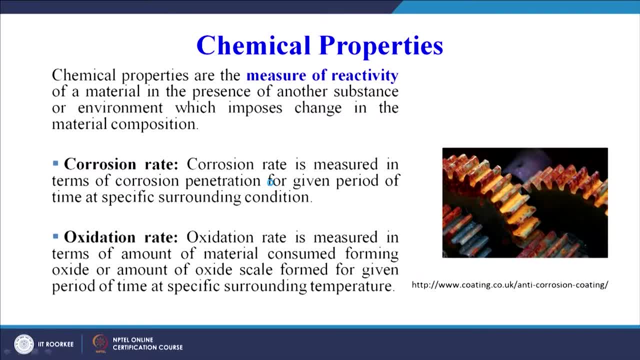 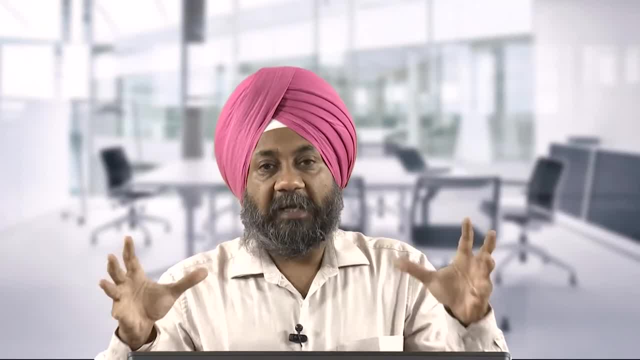 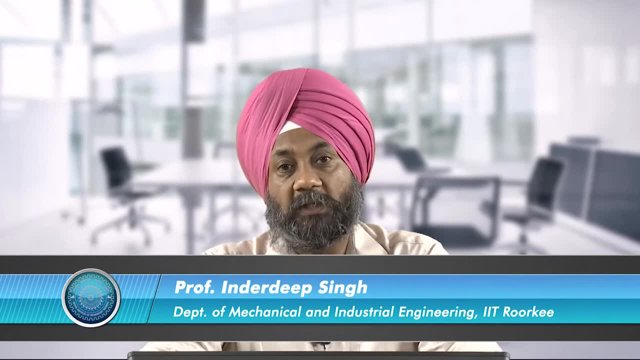 So, similarly, let us now have a basic idea of the various properties. we are not going to discuss each and every property in detail, Because this is a very, very exhaustive topic, and even on materials, As well as metallurgy, as well as materials engineering, there are number of other courses. 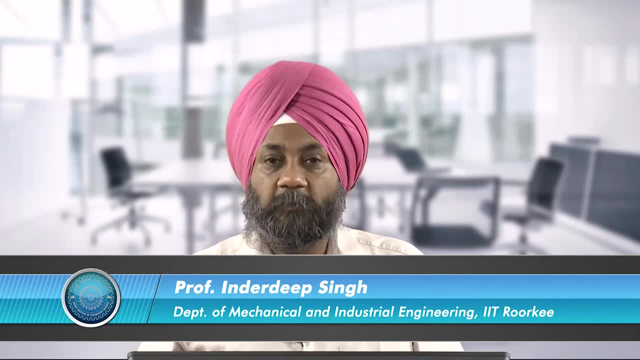 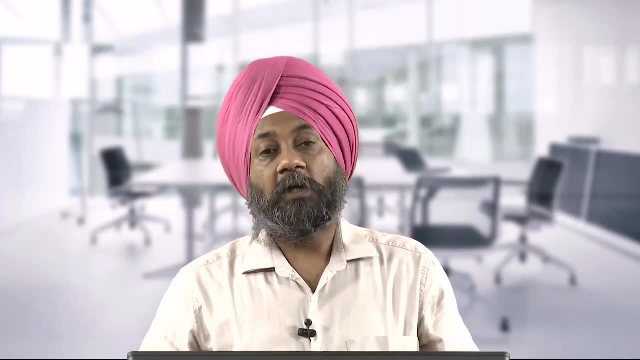 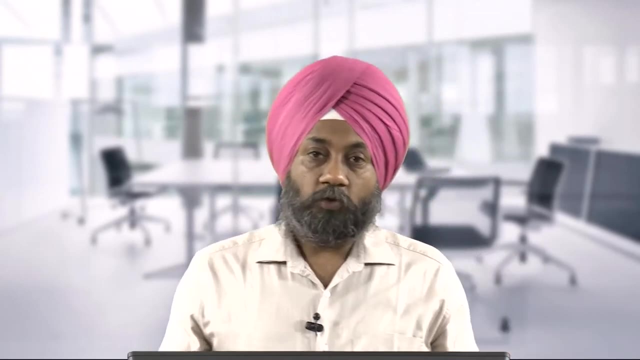 which focus in detail only on the aspects- various aspects- of materials and their application. So our focus is primarily limited to the understanding of the basic idea about the materials from the product design point of view. So our focus is on designing a product and what parameters we must keep in mind, while 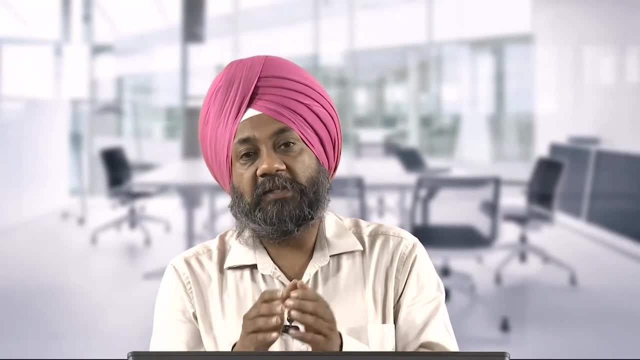 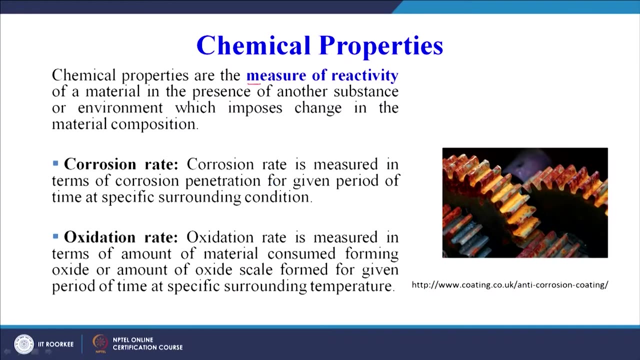 we are finalizing The process as well as we are finalizing the material for our product. So the chemical properties are the measure of reactivity- very, very important, because in corrosion we see how the material is going to react to the environment during the service. 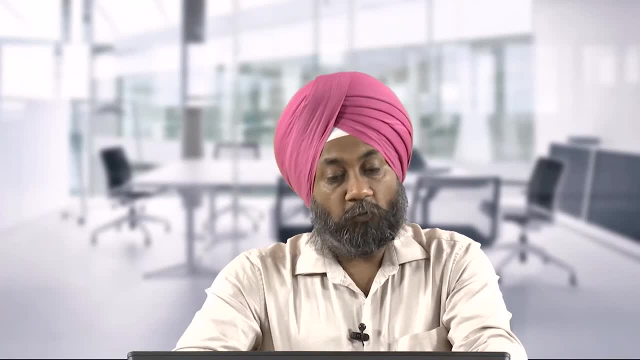 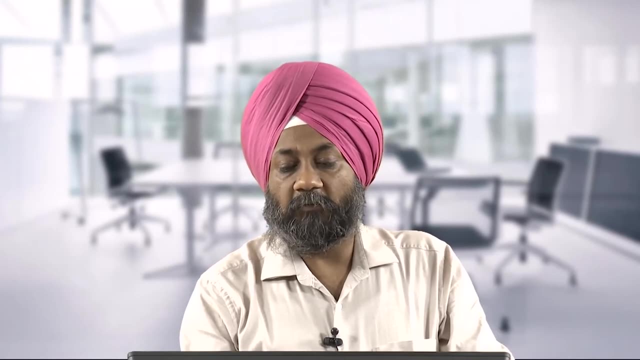 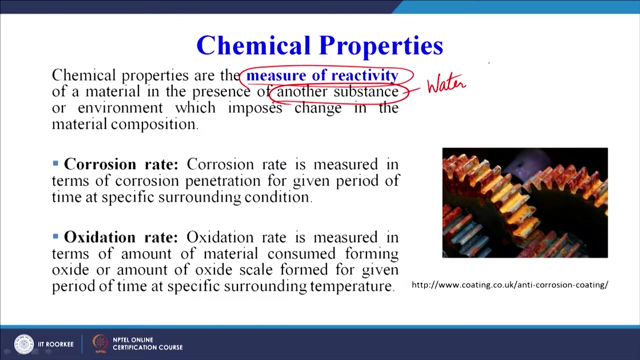 period. So that is the measure of reactivity of a material in the presence of another substance. So in my example, if you remember, the another substance I have taken was water. Under water application I have taken for corrosion or environment which imposes change in the material composition. So the microstructural changes may also take place when the material is exposed to different types of environment or it comes in contact with different substances. So that is the measure of its reactivity. So what is corrosion rate? corrosion rate is measured in terms of corrosion penetration. 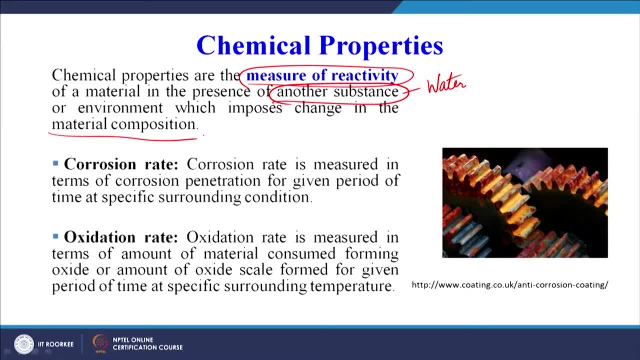 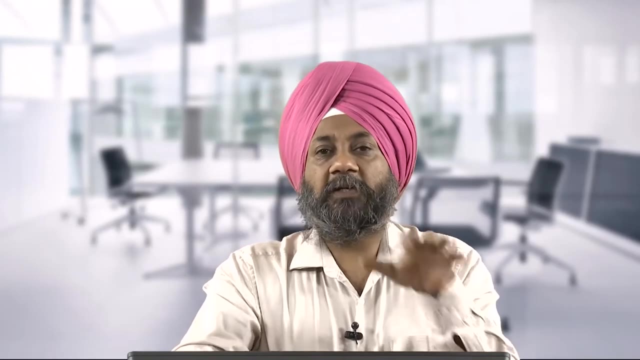 for given period of time, at specified surface Corrosion rate. So at specified conditions. when the product is used, how it is going to react to the penetration or the penetration for a given period of time. So, for a given period of time, maybe 6 months, maybe 1 year, how much corrosion penetration? 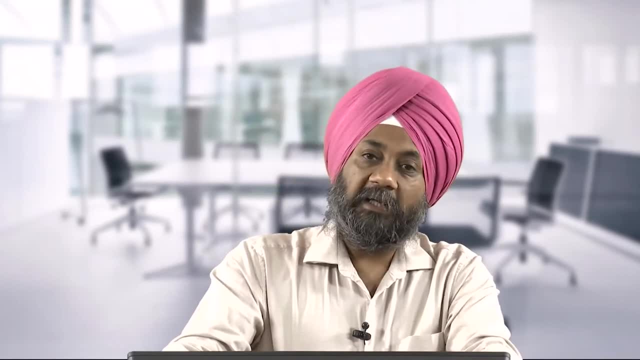 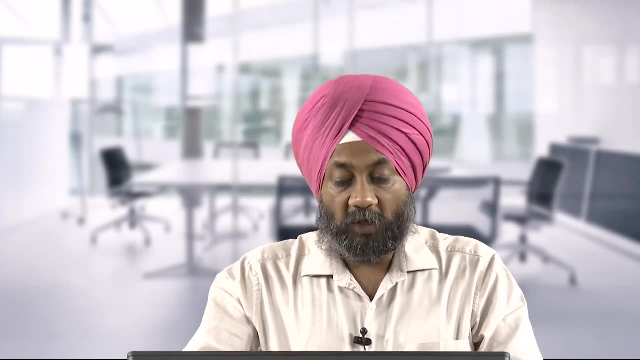 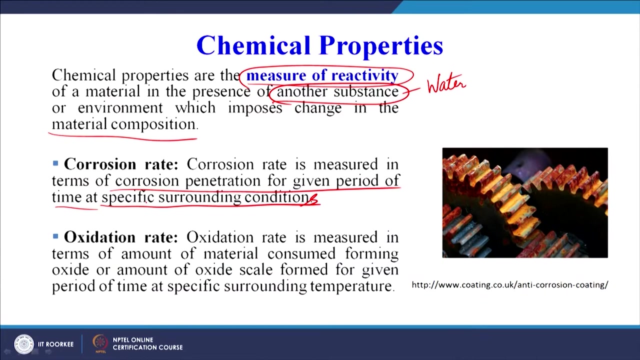 has gone into the material. that is the indication or the measurable quantity we call as the corrosion rate. Similarly, the oxidation rate. Oxidation rate is measured in terms of amount of material consumed forming oxide or amount of oxide scale formed for a given period of time. 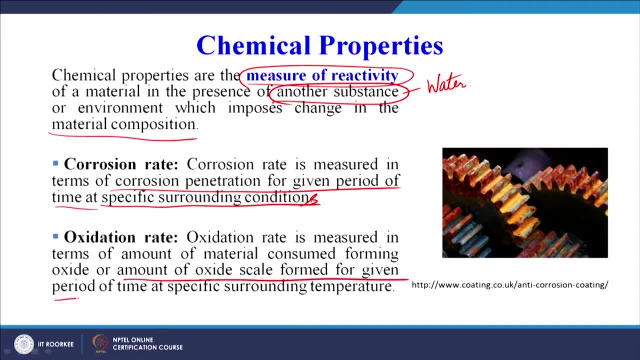 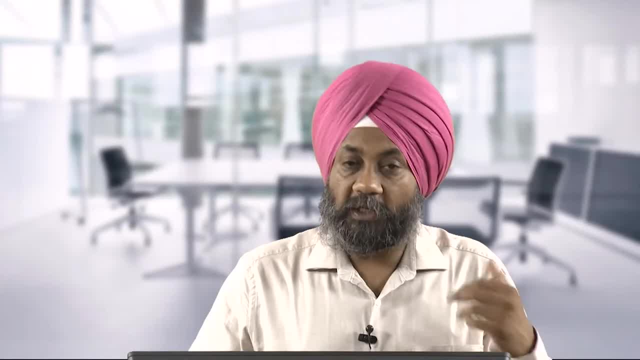 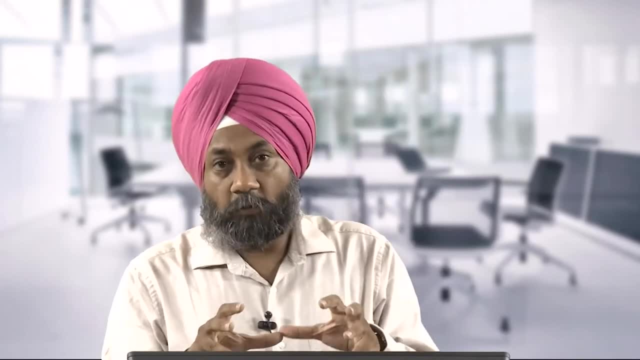 We can say the amount of oxide scale formed for a given period of time at specified surrounding temperature, So we can calculate the oxidation rate. we can calculate the corrosion rate for a material and we may not be interested in calculating as a product designer, but we may look for. 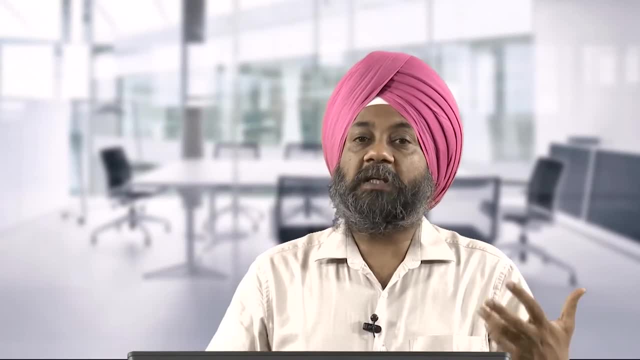 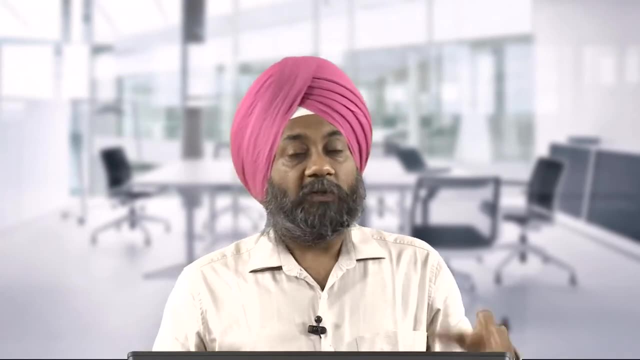 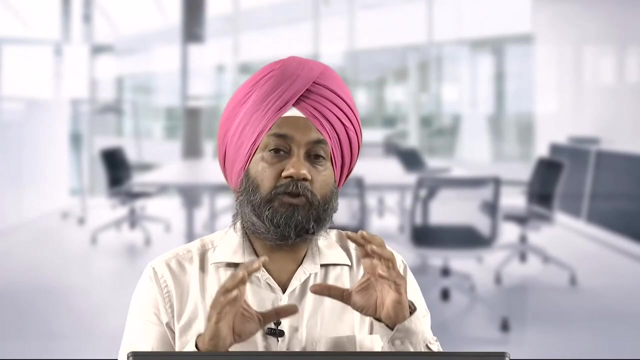 the oxidation rate, it may be available for the material that we are suggesting. So there are 2 different thoughts that are available or that we must keep in mind. If we are suggesting a completely new material for a particular application, we must find out, we must do research on finding out the oxidation rate or the corrosion rate for that. 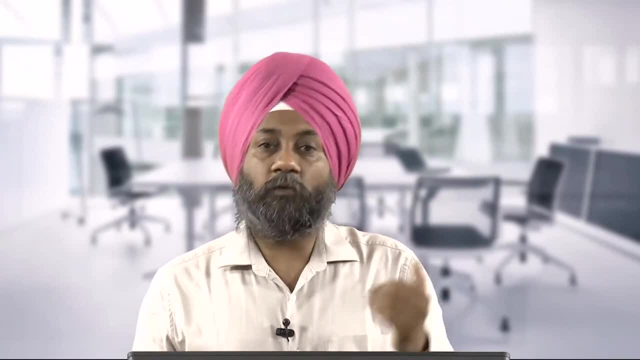 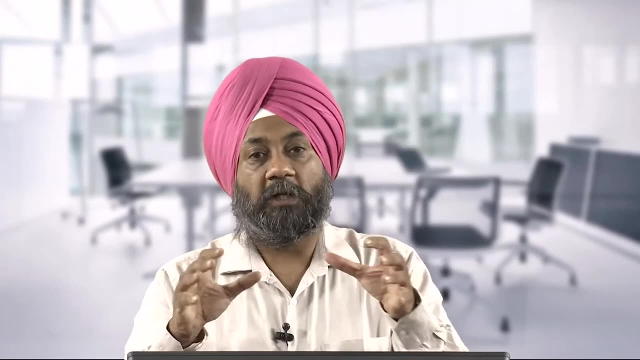 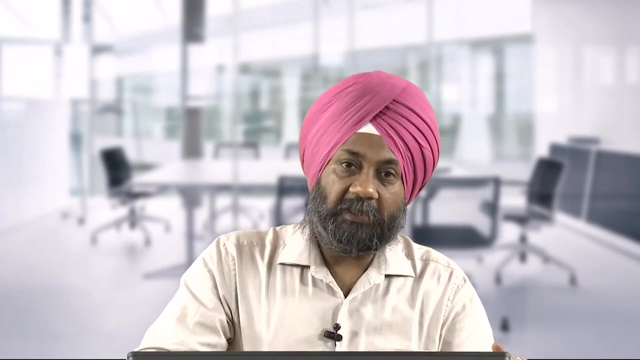 material and then specify that. what is the corrosion rate if it is beyond a particular value. So we must suggest the maintenance procedures, the service procedures for that material or the product during its service life. But if we are using a standard material which is in use for the last 50,, 60,, 70 years, very 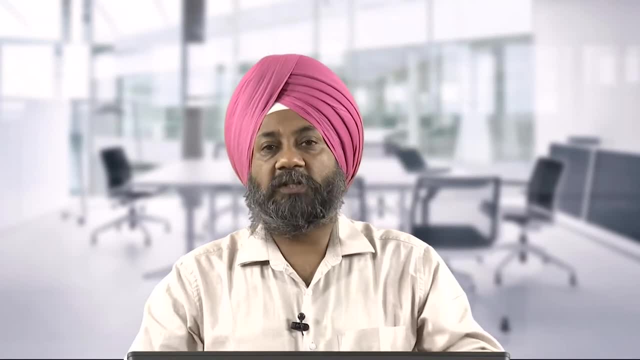 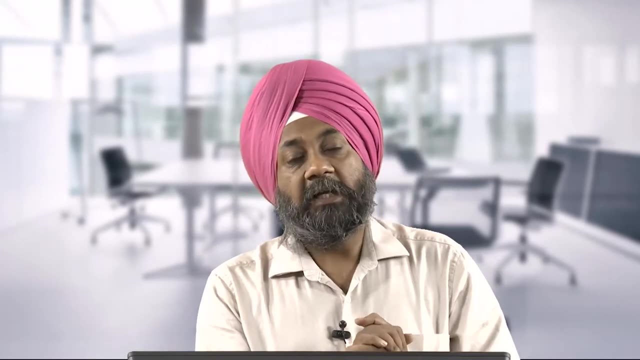 easily we can get the data related to the oxidation rate, related to the corrosion rate of that material. So if the material is a standard material, we can very easily get this data. if we are proposing a new material, We must try to do research, Okay. 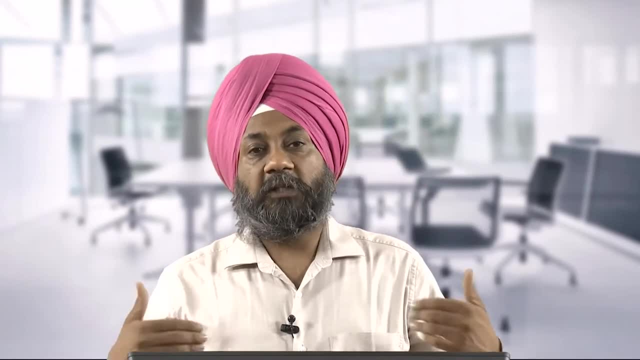 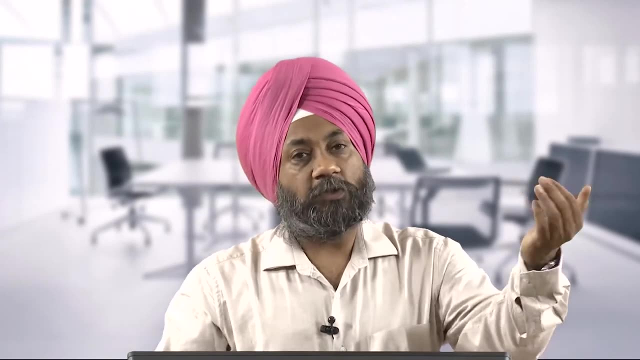 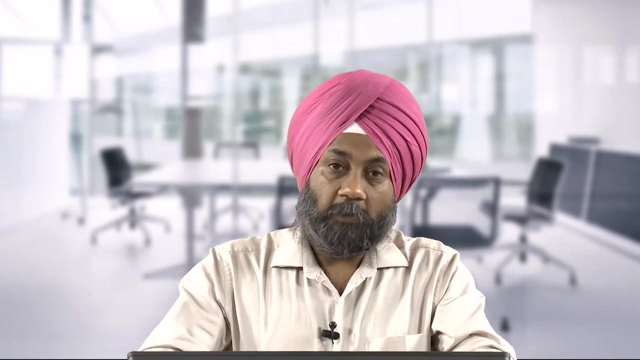 We must try to do research and find out these properties before suggesting the use of this material for a particular application, For example the underwater installations. if we are suggesting a standard steel, we must look for its corrosion rate and oxidation rate from the standard handbooks. 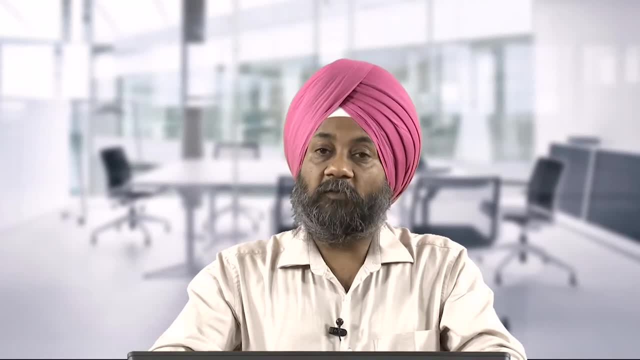 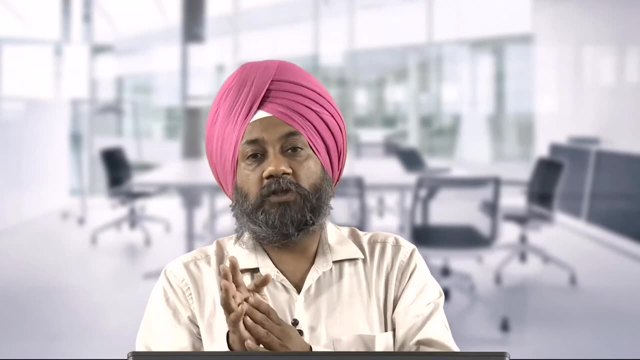 But if we are suggesting a use of a composite material for underwater application, we must try to find out that how it will corrode, or how the fiber, reinforced plastic or a composite material will corrode, How it will react to the water which may be under freezing conditions. 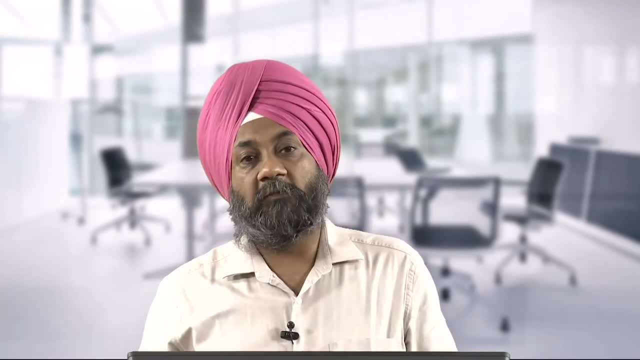 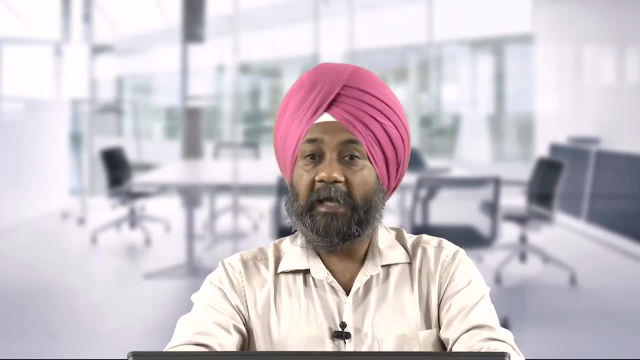 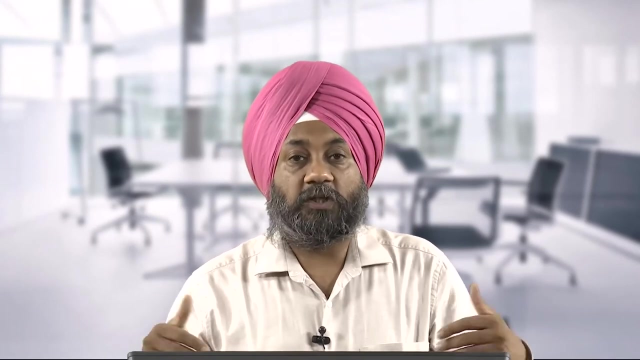 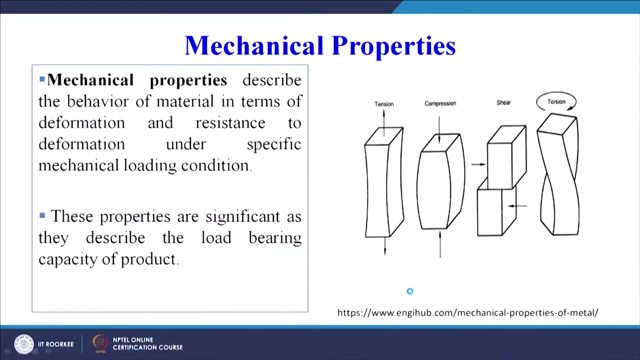 So how that reaction will take place and how the material will behave under those specific application area or under those specific environmental conditions, that has to be found out before suggesting a particular material for the underwater installations. This is just one example that I have taken. Now. the other important properties are the mechanical properties. 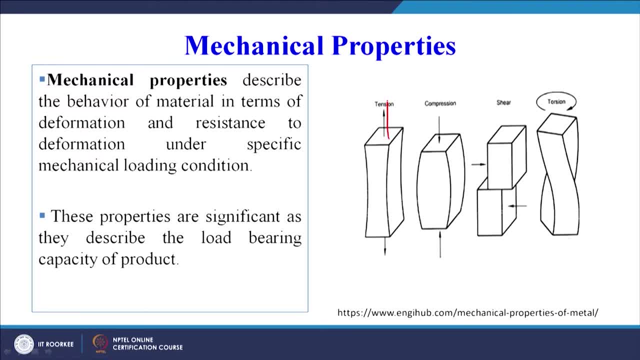 So we can see with the help of example: this is the behavior under the tensile load, the behavior under the compressive load, the behavior under the shear type of loading and the torsional loading. So this is the behavior of a material under applied loads. that how the material is going. 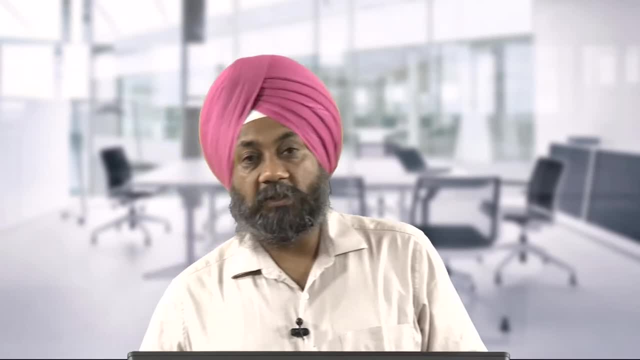 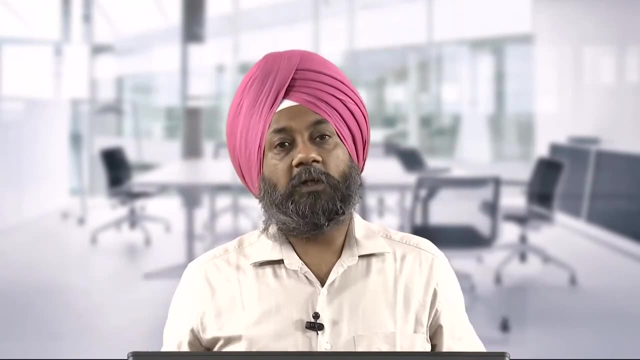 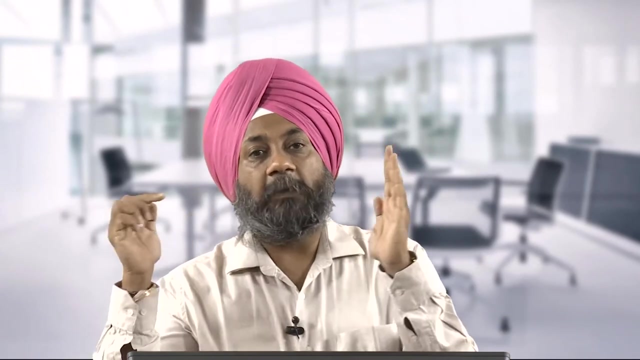 to behave. One of the most important applications that we can see here is the bullet proof applications or the bullet proof materials. Okay, We are making a bullet proof helmet or we are making a bullet proof jacket. So there has to be this investigation that when projectile or a bullet is coming and 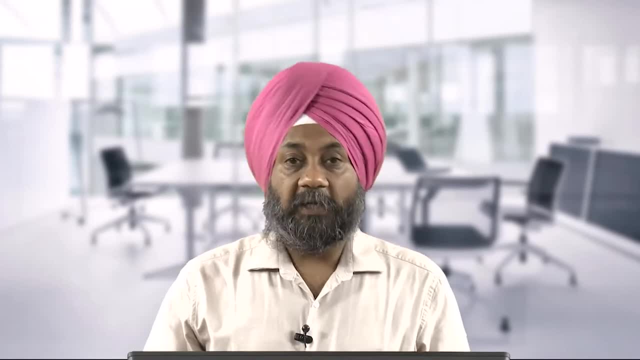 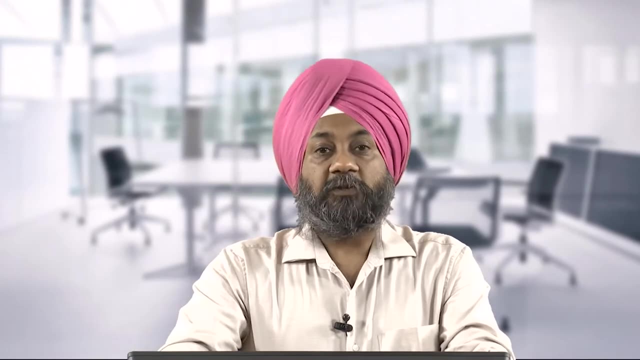 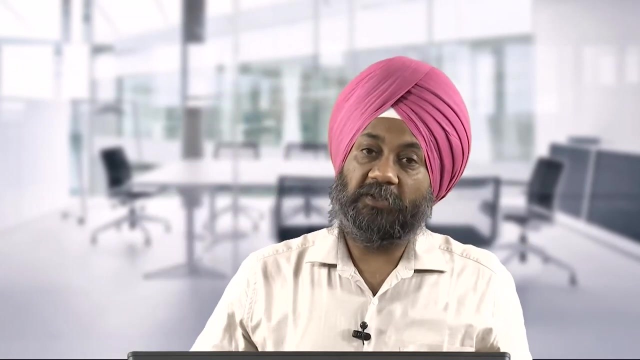 hitting the material, how the material will behave. It must have good impact resistance, So that impact resistance is also a mechanical property. Suppose the material is getting stretched, maybe we can say the mechanical properties of the rods that we use for RCC structure. Or another example where we must know that what is the tensile strength, what is the compressive? 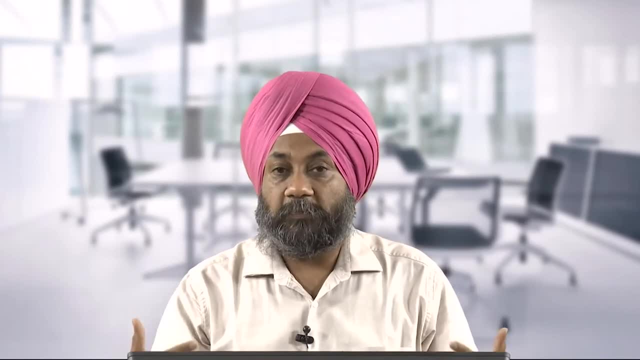 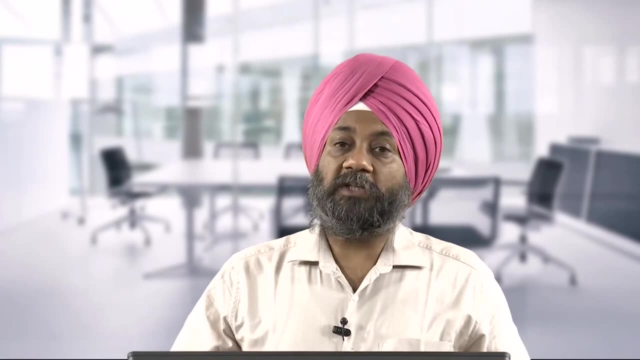 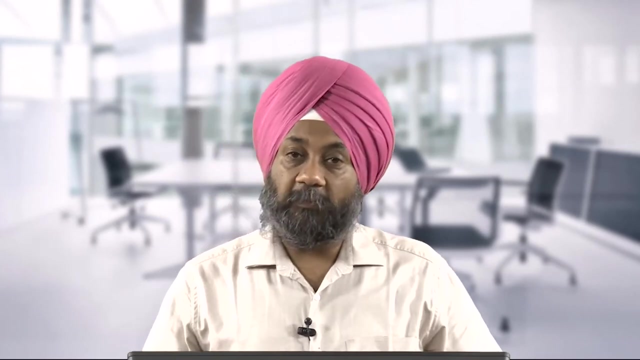 strength of the material. There can be number of examples where the mechanical properties play a very, very important role, a very, very integral role, during the product design process. We must know that, what type of loads the material can bear, before suggesting that material for a specific application and, moreover, whenever we are making structures or for structural 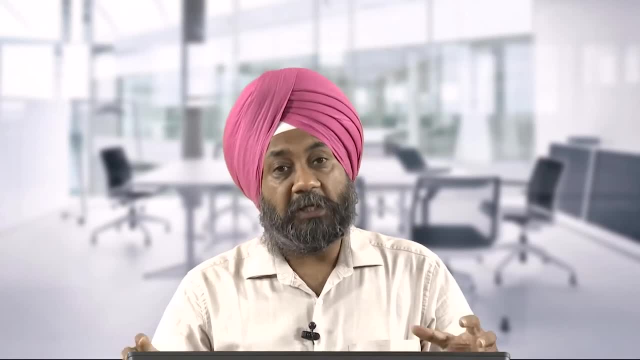 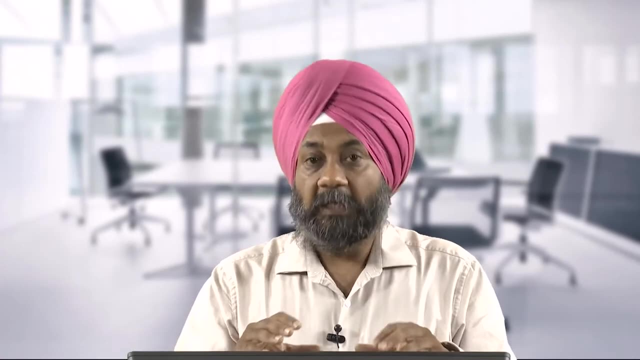 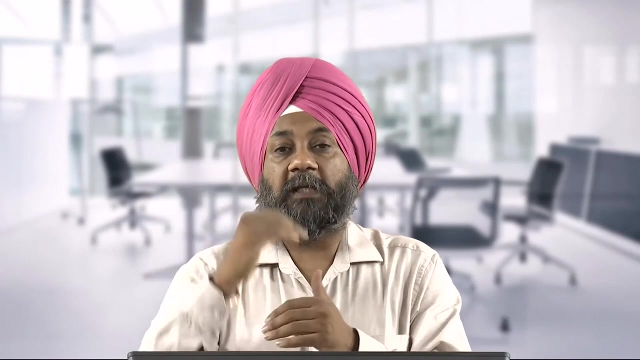 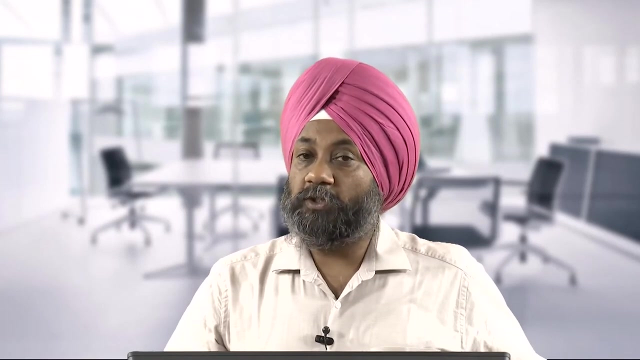 analysis, different type of material is being used. we need to do the standard tests to find out the properties of that material, So that the material passes or surpasses or overcomes, or maybe it has better properties than the specific requirement. So we have to always keep in mind the factor of safety also while proposing the use of. 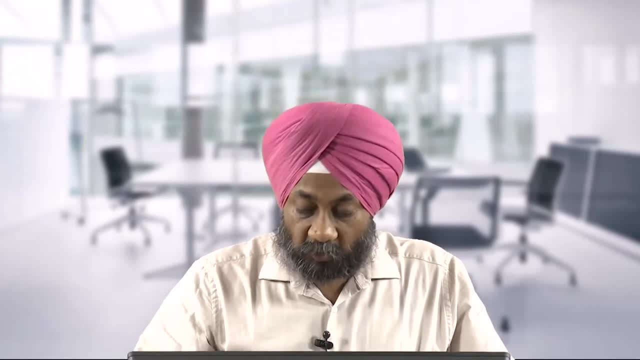 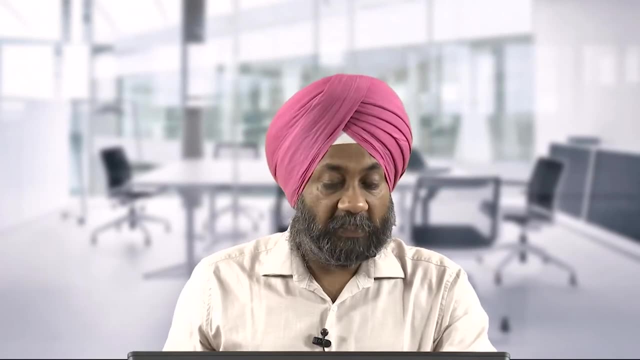 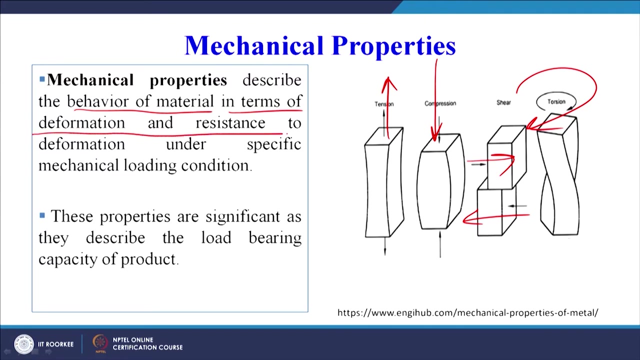 different types of material for a specific application. Let us see the mechanical properties. I have tried to explain with the help of an example. now let us see what is given in the slide. So the mechanical properties describe the behaviour of material in terms of deformation and resistance to deformation under specific mechanical loading. 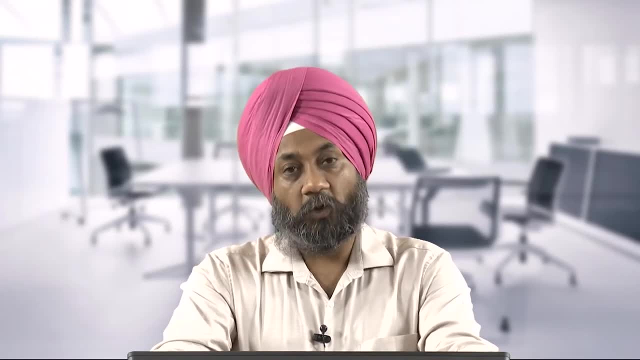 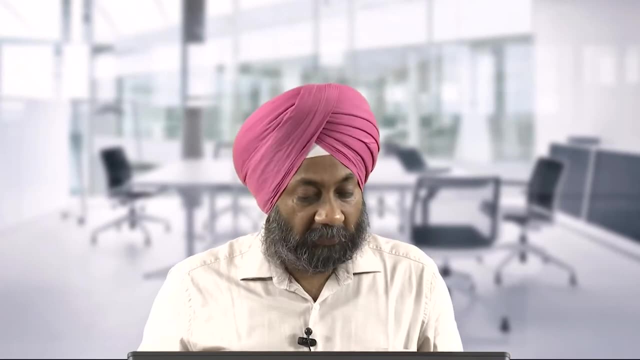 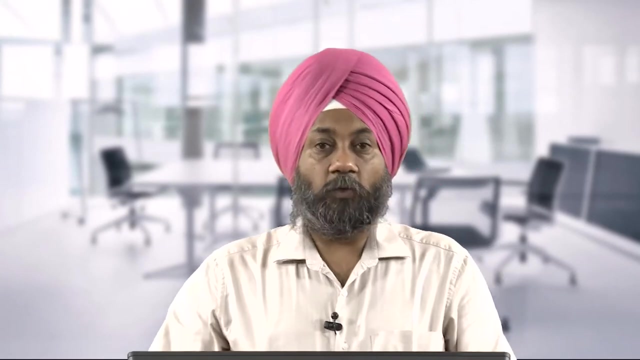 So when the material is subjected to different type of mechanical loads, how it is going to behave. that is going to define the mechanical behaviour of the material. These properties are significant as they describe the load bearing capacity of the product. So we need to understand that these properties are important because they define the load. 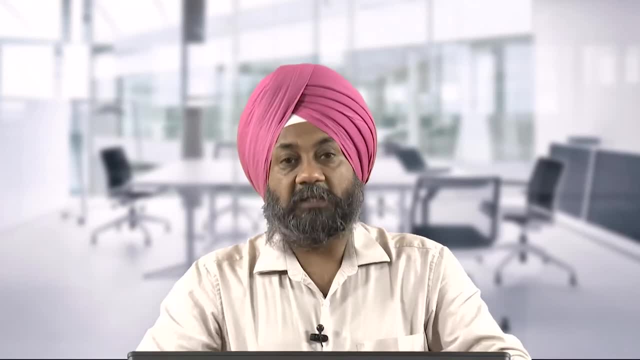 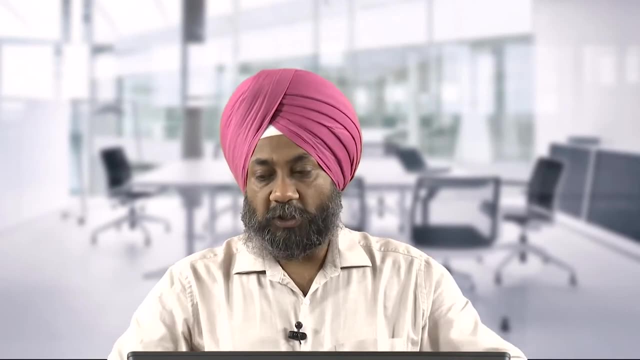 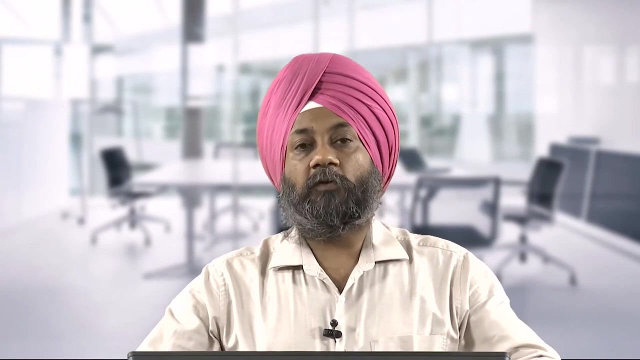 bearing capacity of a product. Now let us take an example of this dice. this is a wooden dice and there is a console panel here. this has a dead weight, So this dice has to have the mechanical property to take the load of this dice. Sometimes I may be standing like this, so I am also putting some weight on the dice. 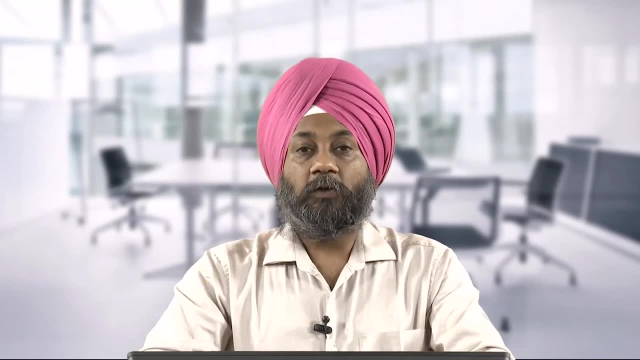 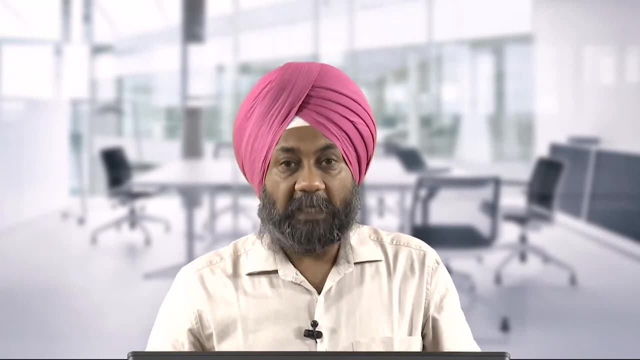 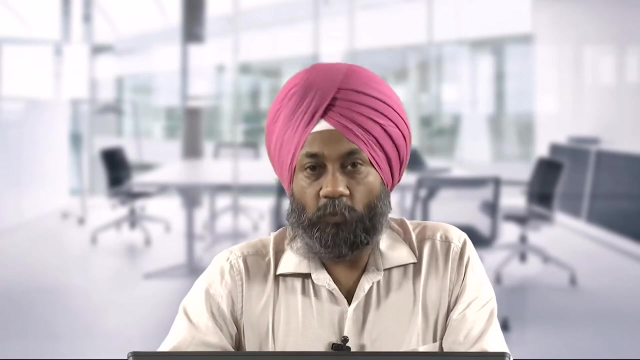 So this dice must have the mechanical property to take that type of load that is being exerted on it, plus a factor of safety. I may not be the most heaviest person who is applying the load here. There may be other people who may exert more load, and this console may be changed by another. 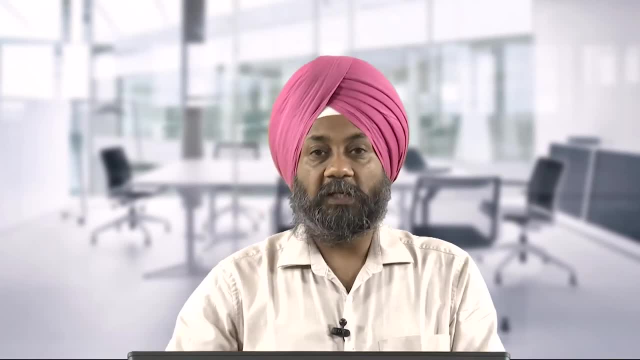 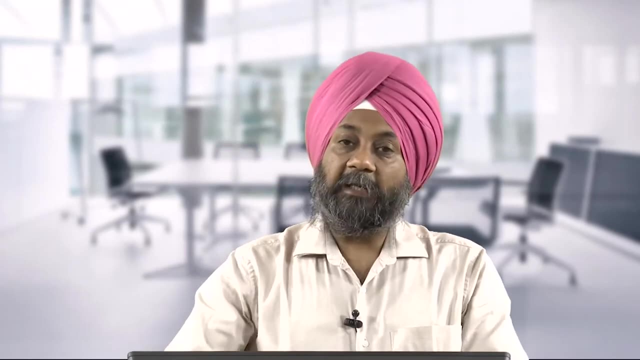 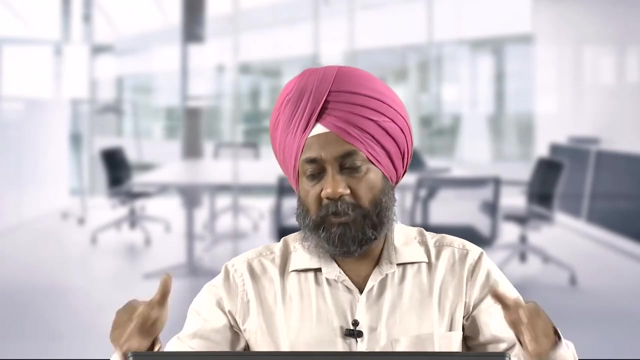 display which may be heavier than this. So we have to see That this product must have the load bearing capacity for which it has been designed. and if suppose we keep a material which is having much more loading or much more weight, So this may also fail under that type of load. 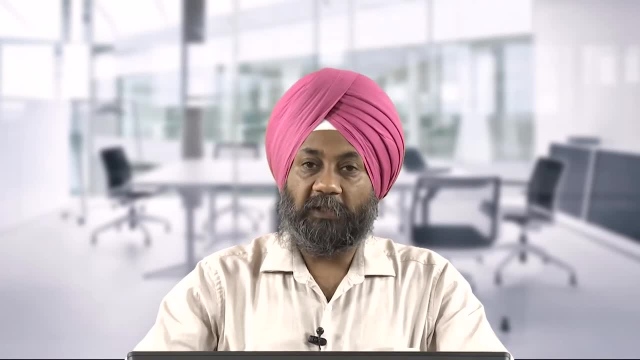 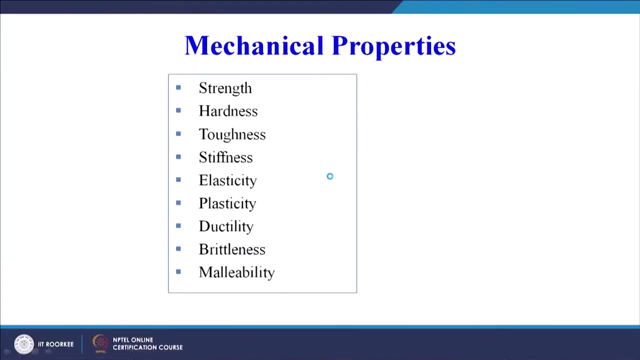 So we have to see the load bearing capacity of the material before proposing its use for specific applications. Now, these are the various mechanical properties There. There are other properties also. Some of these properties we can see here. This is strength, hardness, toughness, stiffness, elasticity, plasticity, ductility, brittle. 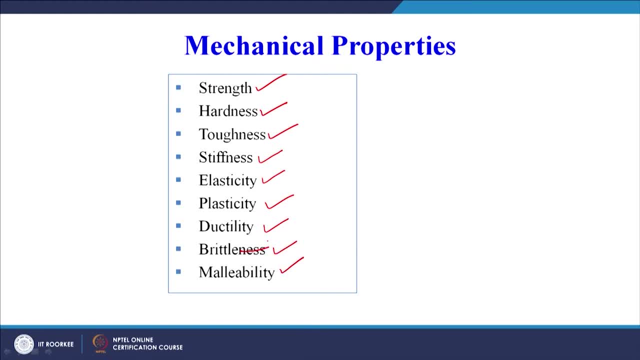 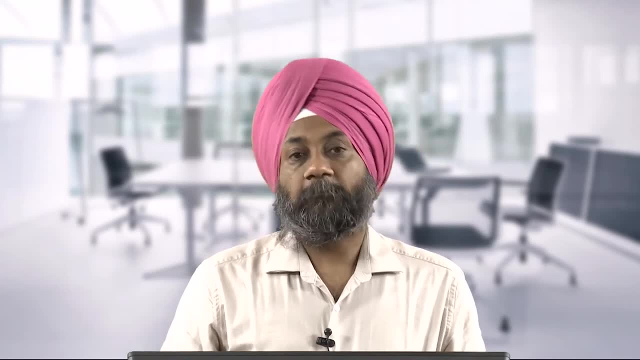 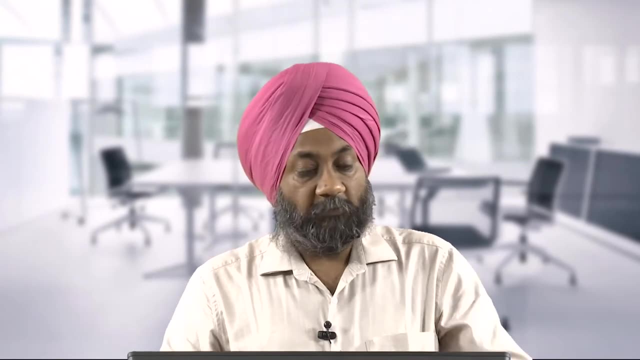 behavior malleability. So we have different types of mechanical properties which define the mechanical behavior of an engineering material. So we cannot go into the detail of each one of these, So let us quickly see the 3 important definitions. Strength is the property that enables an engineering material to resist deformation. 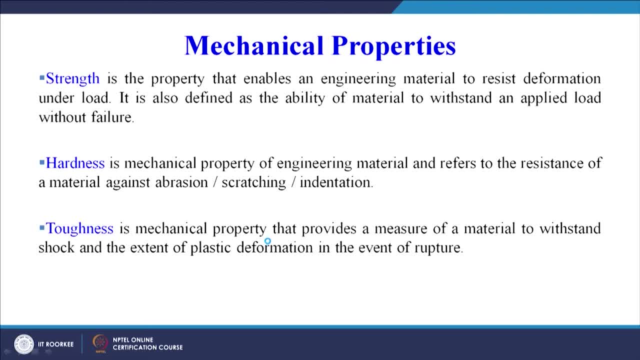 under load. It is also defined as the ability of the material to withstand an applied load without failure. Hardness is the mechanical property of an engineering material and refers to the resistance of a material against abrasion, scratching and indentations. So hardness is related to resistance to abrasion, scratching and indentation. 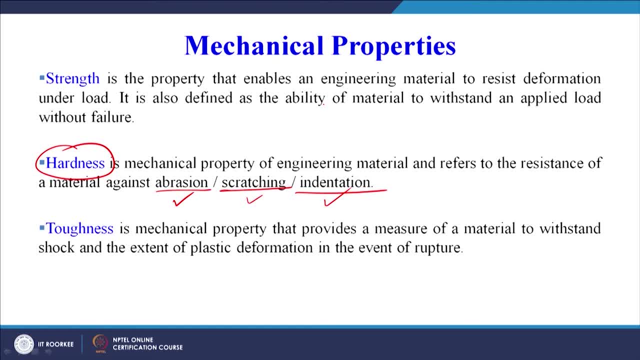 Soju Kyochiku Hakichi Soon K TA. strength is related to ability of a material to withstand an applied load without failure. Toughness is the mechanical property that provides a measure of a material to withstand shock, so toughness is related to shock absorption, or withstanding the shock and extent of plastic. 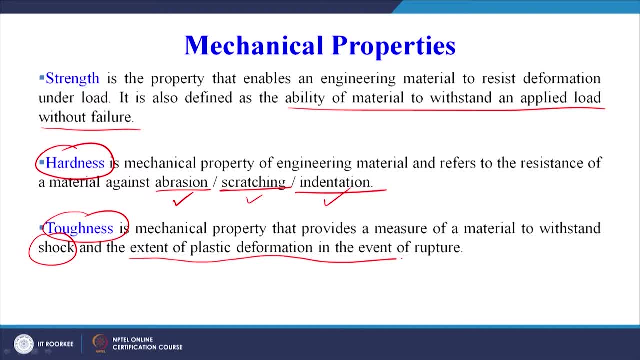 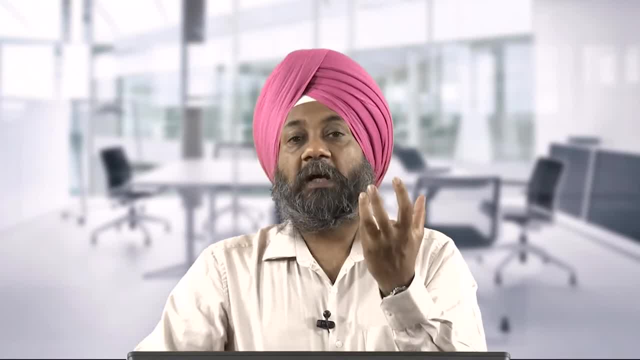 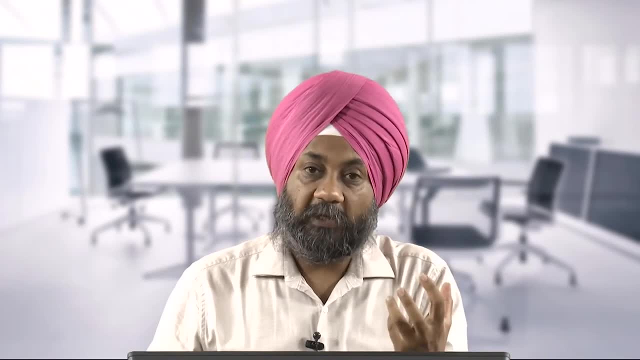 deformation in the event of rupture. So how much plastic deformation can take place before the final failure? so we are just giving you a hint about these 3 properties, But the list is very, very exhaustive. of material may be defined or characterized for its mechanical 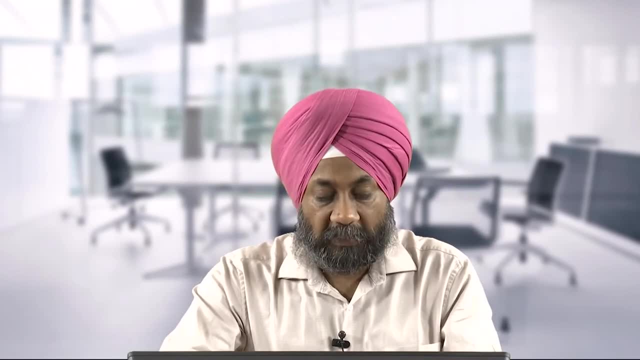 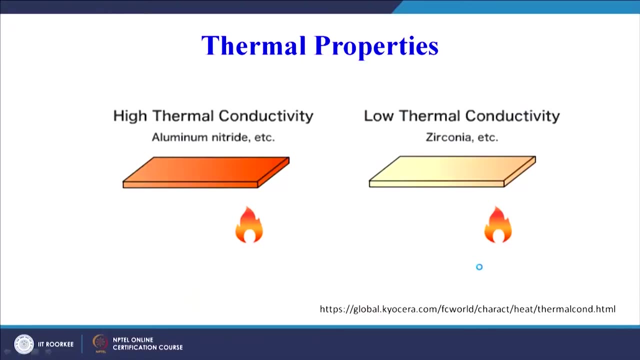 behavior using large number of mechanical properties. Now, finally, we can go for the 4th category of properties, which are the thermal properties. so high thermal conductivity example is given, so it has high thermal conductivity. low thermal conductivity example is given here, So we can see from the picture also, when it is getting heated, how the heat is getting. 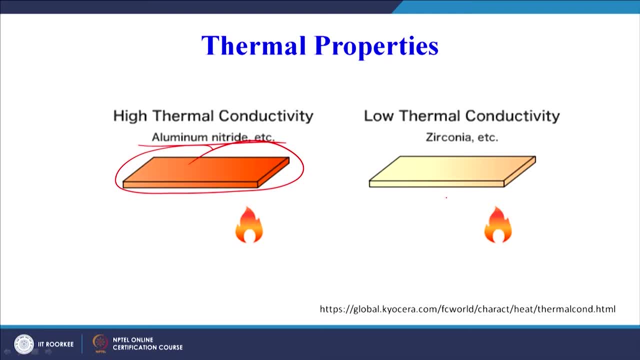 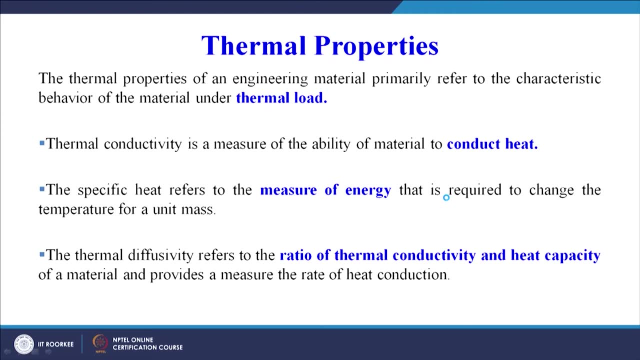 conducted in the material here less conduction because of the low thermal conductivity. So what are the thermal properties? let us see. thermal properties of an engineering material primarily refer to the characteristic behavior of the material under thermal load. So when thermally you are applying, you are giving heat to the material, how it is going. 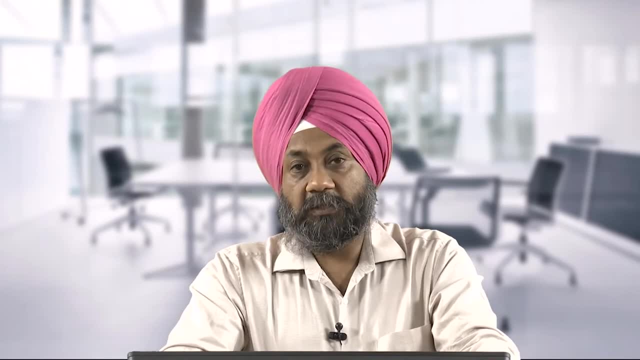 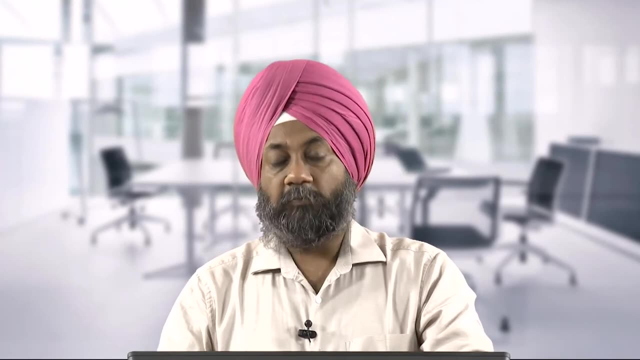 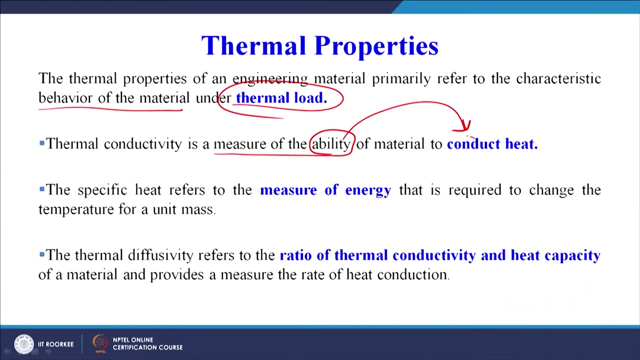 to behave. That is known as the thermal characteristics or behavior of the material. so thermal conductivity is a measure of ability of material to conduct heat. so measure of the ability. Now, what is the ability of the material to conduct heat? that is going to define the thermal. 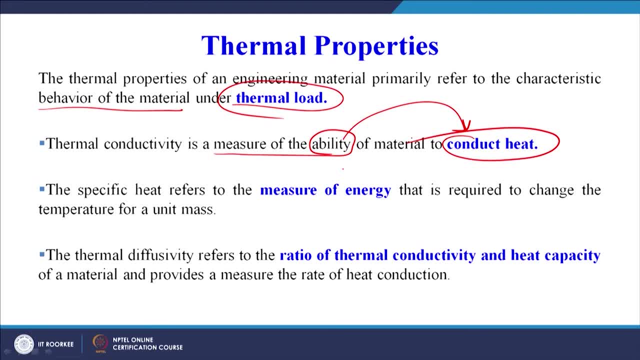 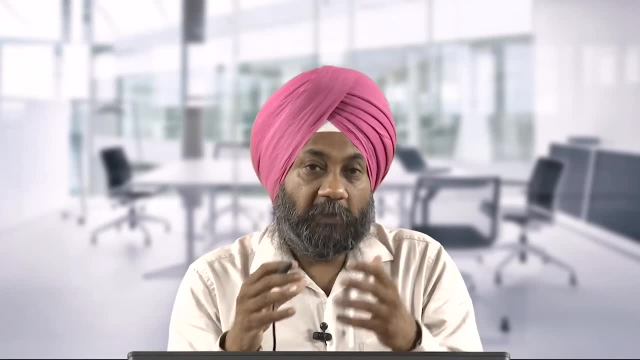 conductivity. The specific heat refers to the measure of energy that is required to change the temperature for a unit mass, So we can have different parameters. So when you are going to design a particular product and then you want to understand that how it will behave when subjected to heat, 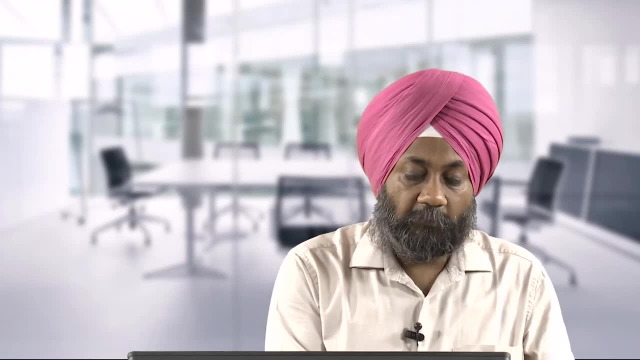 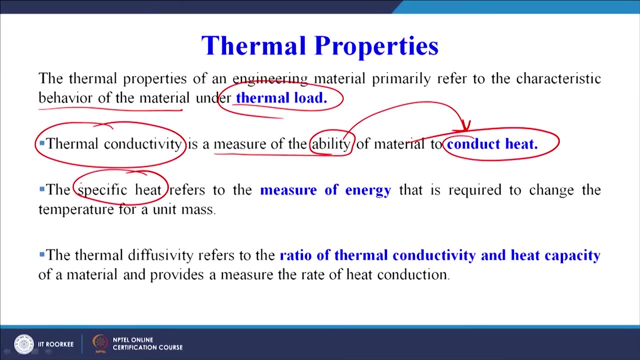 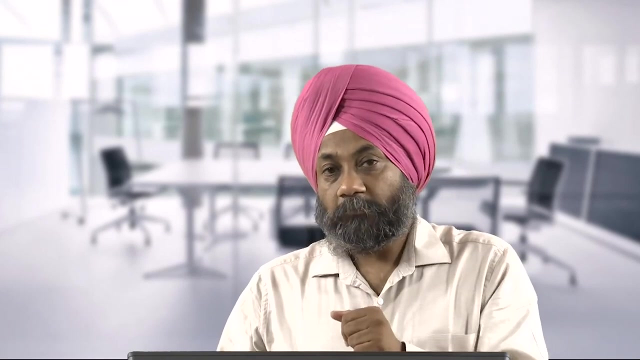 You need to understand few parameters. you need to understand important parameter, that is, thermal conductivity. you need to understand what is the specific heat of the material and these quantities for the material will be available in the tabular form, so we need not worry. 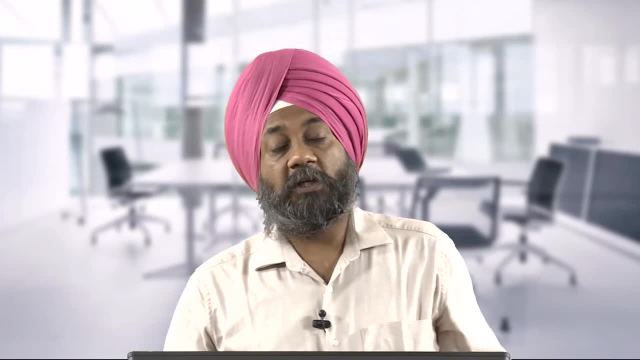 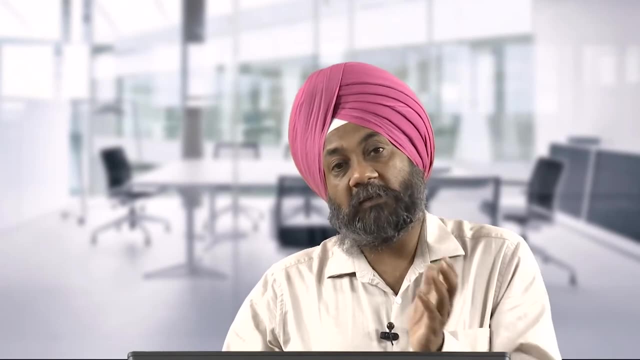 worry that how we will get to know that what is the specific heat of the material, how we will get an idea that what is the thermal conductivity of the material. So this type of data is already available, but as a product designer I must know that. 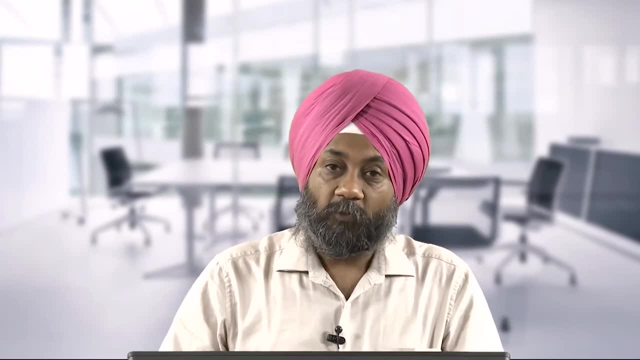 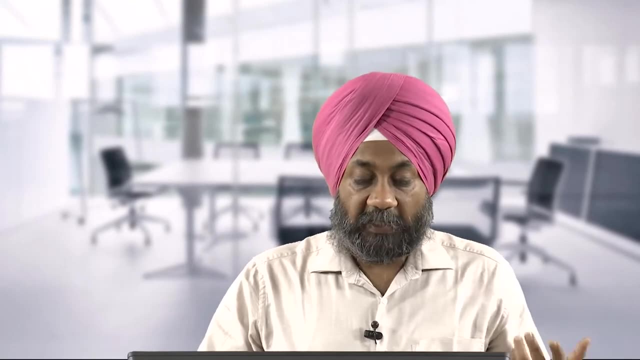 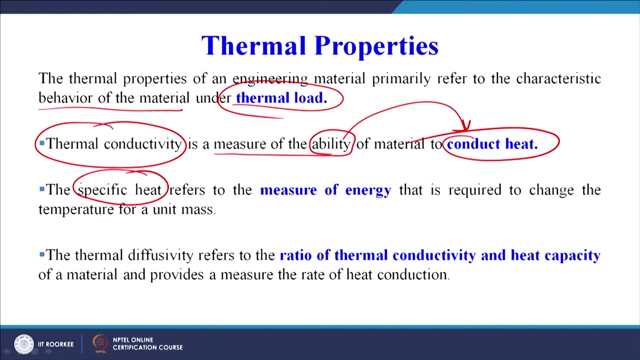 this data is available. I must look at this data while before suggesting material for a specific product application. So what is specific heat? it refers to the measure of energy that is required to change the temperature of a unit mass, So that, therefore, for a specific product where we want to change the temperature of a unit, 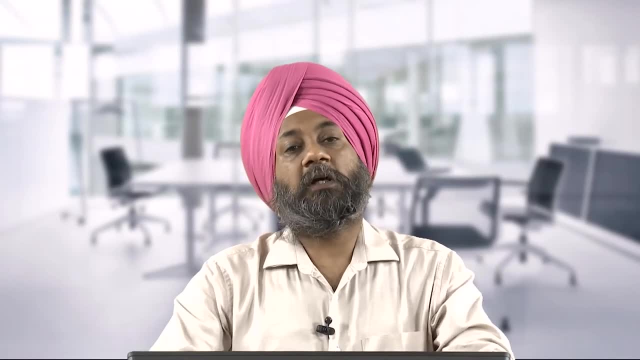 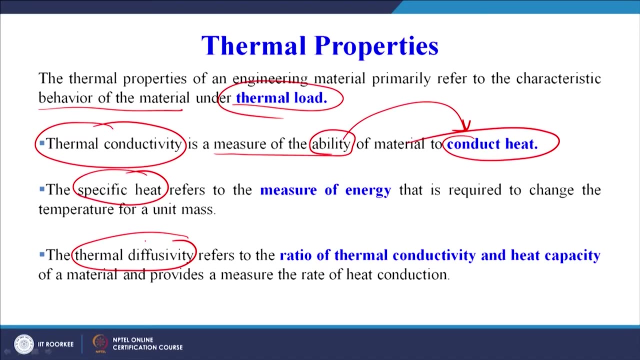 mass. we must know what is the specific heat for a material or of the material. So thermal diffusivity, another property. thermal property refers to the ratio of thermal conductivity and heat capacity of a material and provides a measure of the rate of heat conduction. 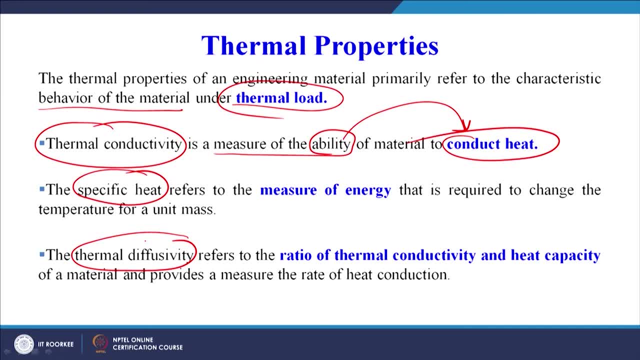 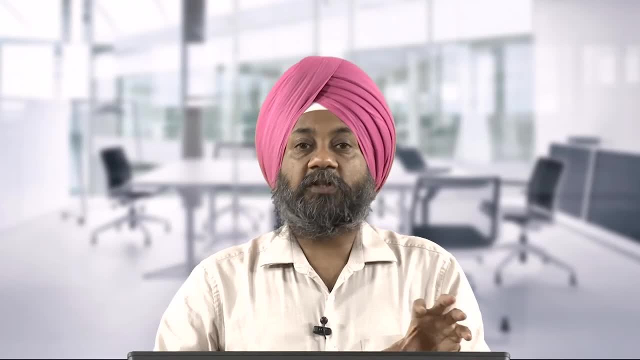 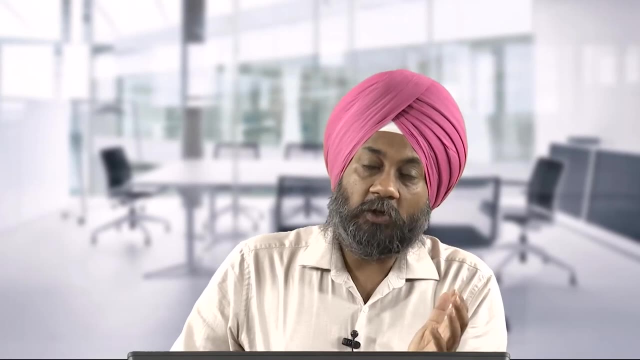 So you have thermal diffusivity. So thermal diffusivity, specific heat, thermal conductivity. then there can be other properties which define the thermal behaviour of any engineering material And as a product designer, I must look into these characteristics or properties which define the thermal behaviour only in those cases where the product is going to be subjected. 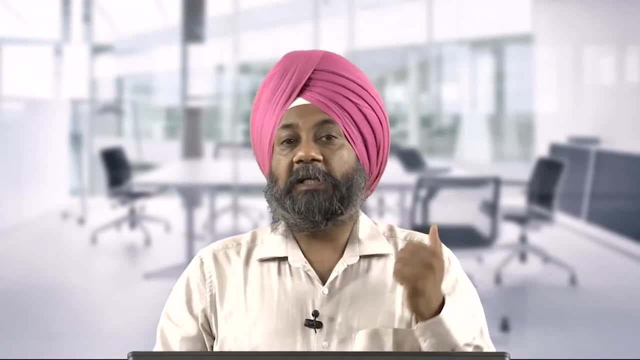 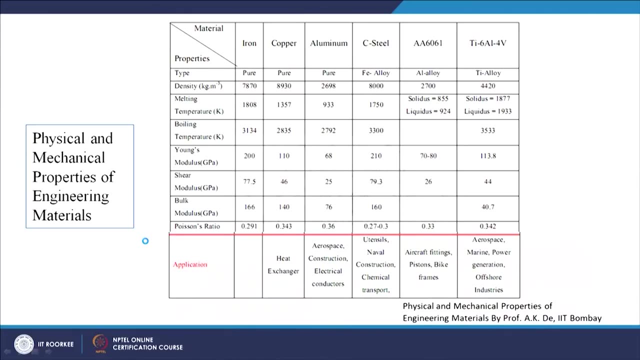 to heating conditions, or maybe high heating conditions. Now, this is the last slide for today. physical and mechanical properties of engineering material. source is also given: physical and mechanical properties of engineering materials by Professor AK Day from IIT Bombay. this is taken from the source: 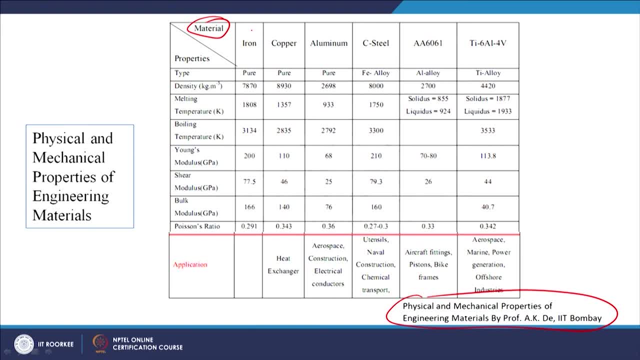 So we can see what are the different types of materials in this direction: iron, copper, aluminium, steel, aluminium 6061, titanium, Okay, 6L4V. So different types of metals and alloys are there, and then the properties are given. 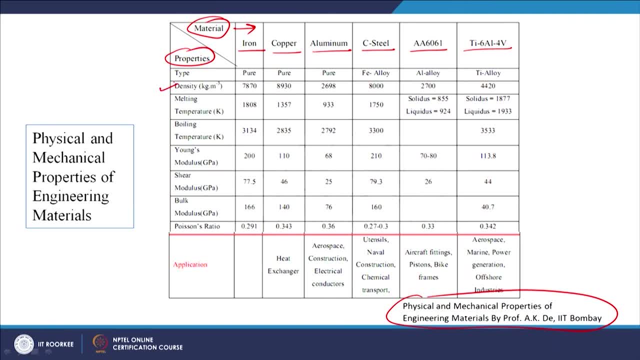 The properties are density. if you remember- today only we have taken an example- density falls under our physical properties. Then the melting temperature is given, boiling temperature is given Young's modulus, which is a mechanical property, shear modulus, which is a mechanical property, bulk modulus, which 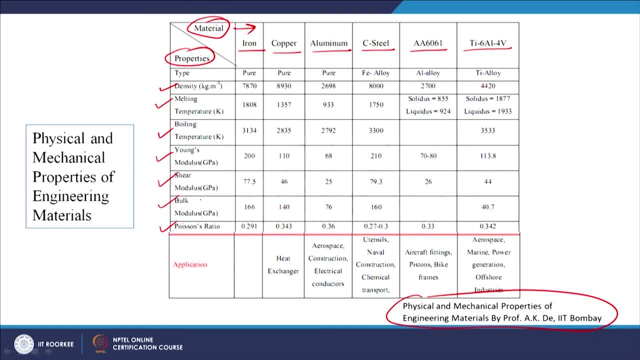 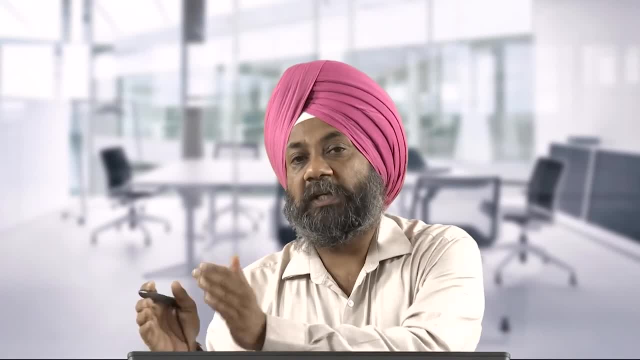 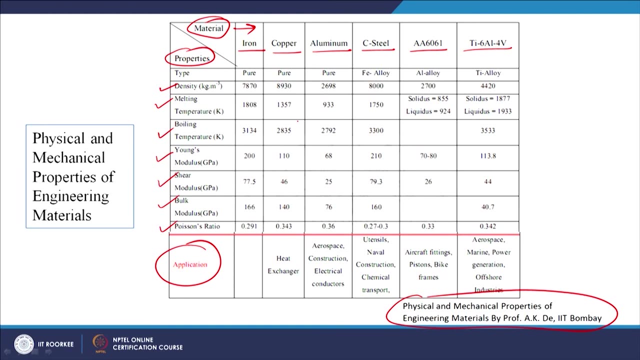 is a mechanical property. Poisson's ratio, which is a mechanical property. So The combination of physical and mechanical properties are given in this table for various engineering materials. and finally the applications are given. So you can see that all the thermal properties are not mentioned here, but copper is used. 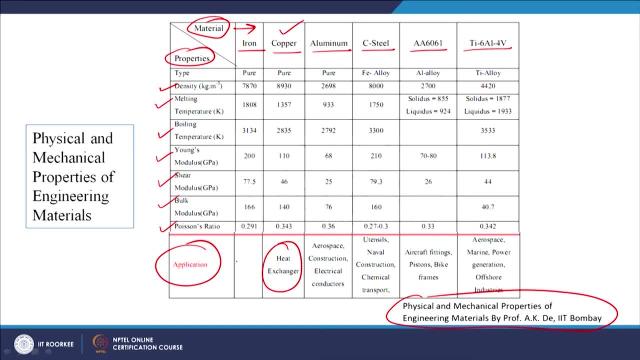 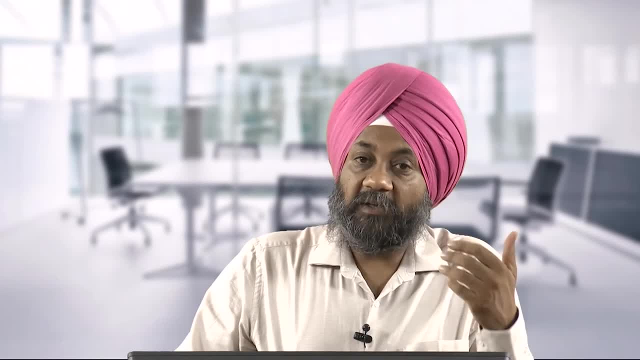 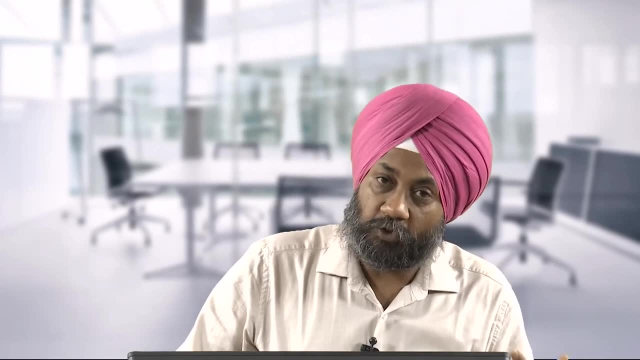 for making heat exchangers. why it is used? because of its good thermal properties. What are the thermal properties that we can look for? We can look for thermal conductivity. We can look for specific heat. We can look for thermal diffusivity. 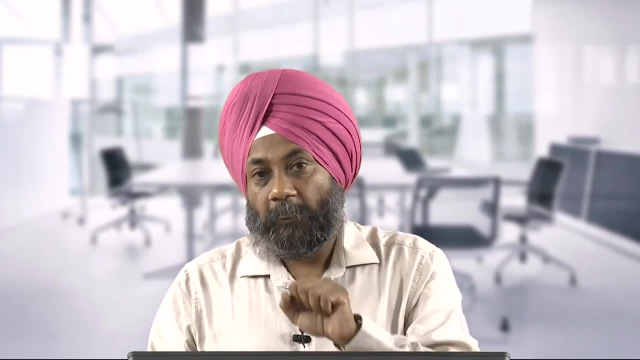 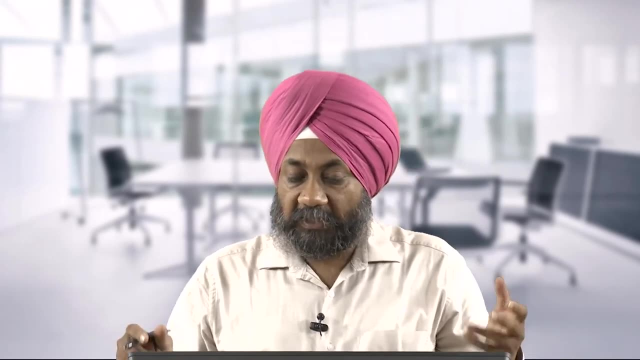 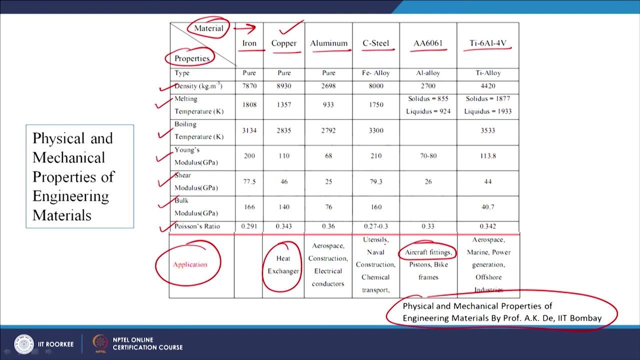 So when we are suggesting an application for heat or for where the temperature is important, we must look for the thermal properties of the engineering materials. Let us take one more example. maybe aircraft fittings. we are taking for this AA6061 material, So we can see that, the mechanical properties, what is the Poisson's ratio, what is the density?